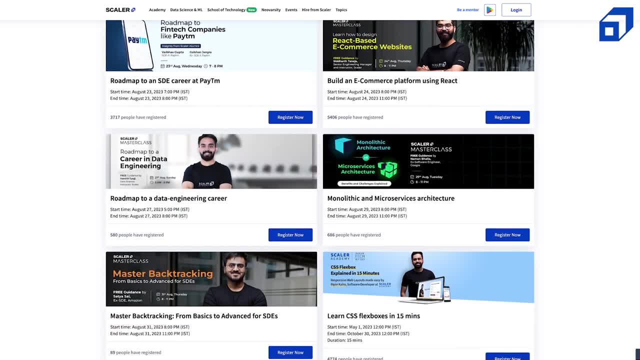 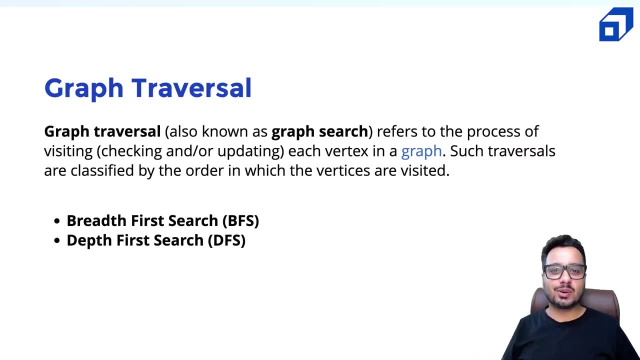 But before we get started, make sure to checkout free masterclasses on scaler's event page to learn from some of the best industry experts. Link is in the description below. Let's begin with the tutorial. So let us talk about graph traversal first. what is actually is a graph traversal? 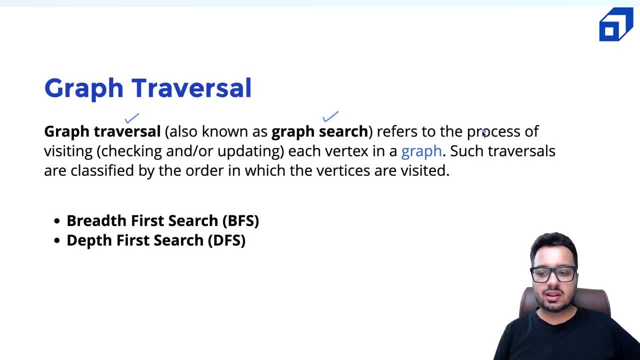 So graph traversal, also known as graph search, is a way or is a process of visiting each vertex in a graph. Such traversal, as I told you, are classified into two types. One is BFS, which stand for breadth, first search. it is a iterative way to traverse the graph. and second one is a recursive way, called depth first. 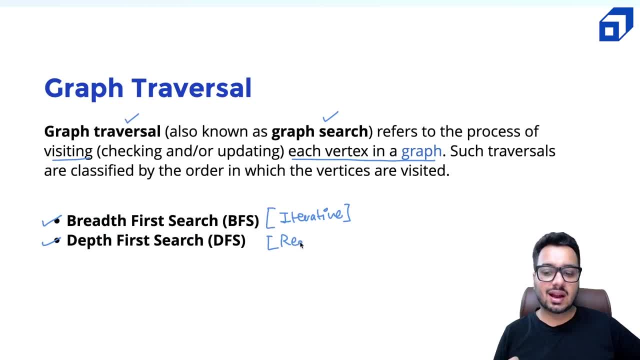 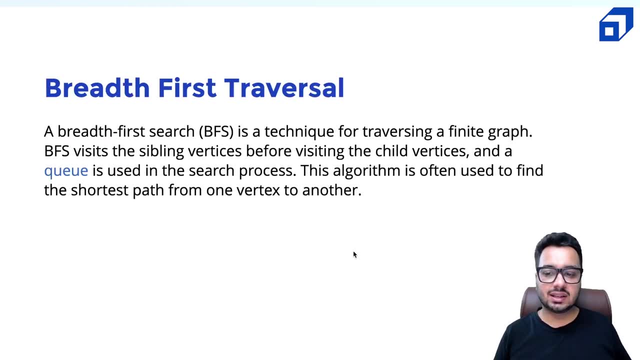 search. in this tutorial, we'll focus on bfs and its applications. so bfs actually has many applications, and one of the most commonly used application is finding shortest paths in undirected graphs. we'll also look at such applications in this tutorial. so let us start talking about bfs. 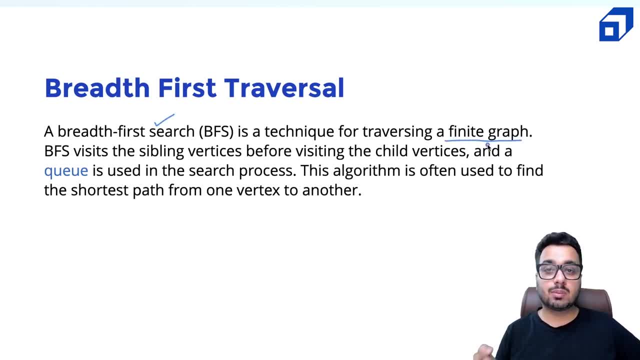 it is a technique for traversing a finite graph. that means the number of nodes in the graph would be finite, and the way it works is it visits the sibling nodes before visiting the child vertices. so what does it means if you have something like a node a and it has children like b and c? 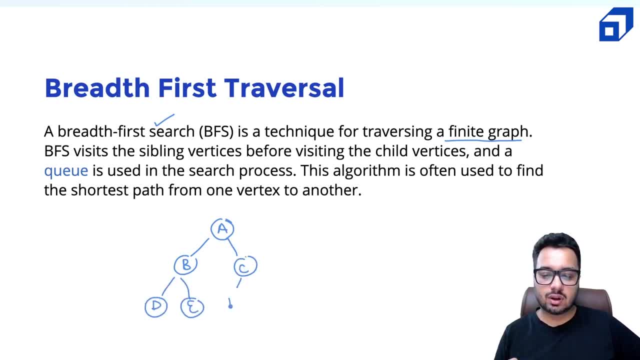 and then you have some children like d and e and so on. the way it works is if you look at in the form of a tree, suppose this graph is a tree. now this is not a tree because i'm added one more edge here. the way it works is it will visit this node. 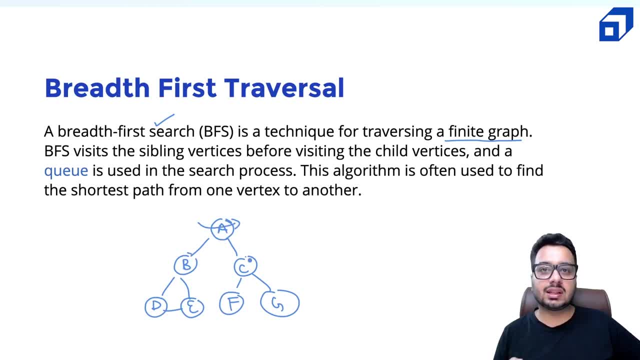 then it will come at b but will visit sibling of b, that is c next. so it will visit b, c, then it will visit d, e, f, g and so on. in a way, if you look at in the form of a tree tree like traversal, it is like a level order, traversal. 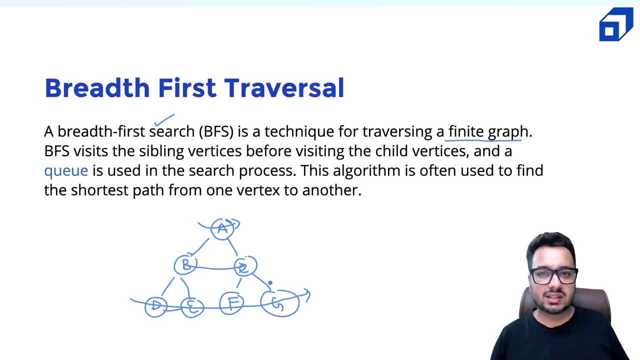 that we have done in a tree, but in a graph it will be quite similar, but there is one catch. the catch is graph contains a cycle. right, we have to make sure that we are not visiting a node which is already visited. for example, from this node one, if you visit two and two is connected with three. 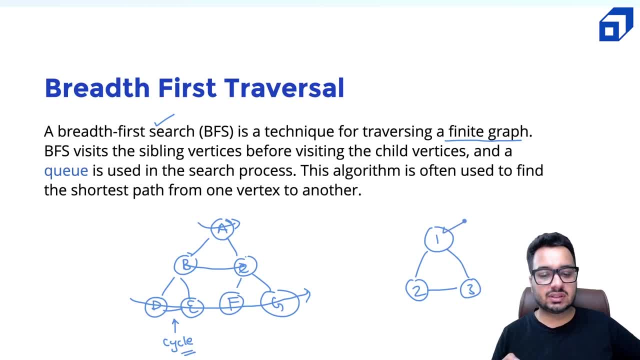 three is connected with one. so there is a cycle. if you say okay, i will visit one, i'll visit children of one, that is two, i'll visit three from three now you cannot go and visit one again, right? so this is something we have to make sure is handled properly by our algorithm before i dive. 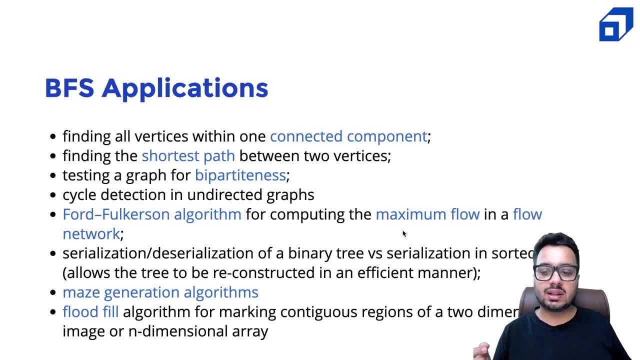 deep into the algorithm or into the code. let us try to understand some applications of bfs. bfs is can be used to find all the vertices within a connected component, so we want to see what parts of the graph are connected. it is also used to finding shortest path between: 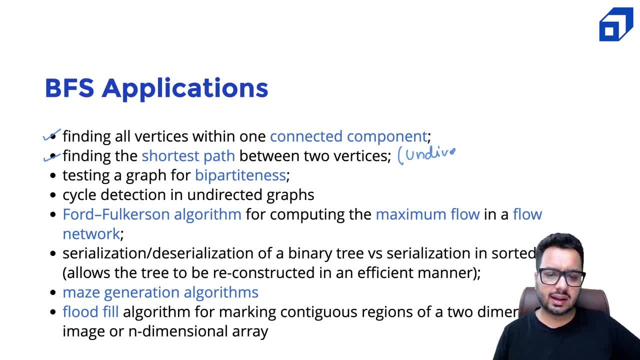 two vertices. in case of a undirected graph, that means all the edges. sorry, unweighted graph, that means all the edges. they have equal weight. there is no weight assigned to any edge. if there is a weight, then we have to use a different algorithm. it can be used to check a graph for bipartness. 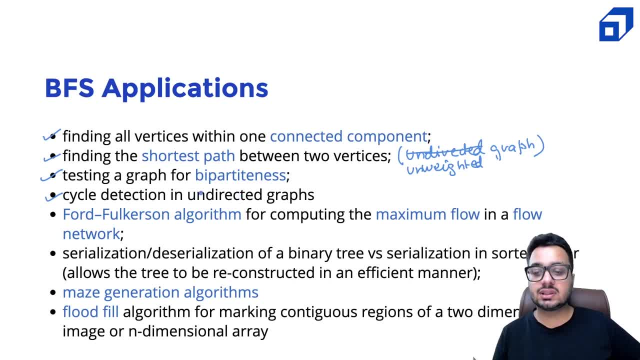 it can be used for cycle detection in undirected graphs. it is also used in ford fulkerson algorithm for maximum flow. it is also used in serialization- deserialization of binary tree. it is also used in maze generation algorithms and it can also be used in algorithms like flood field. there are 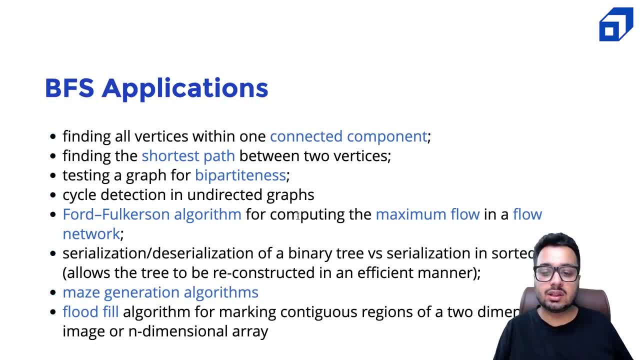 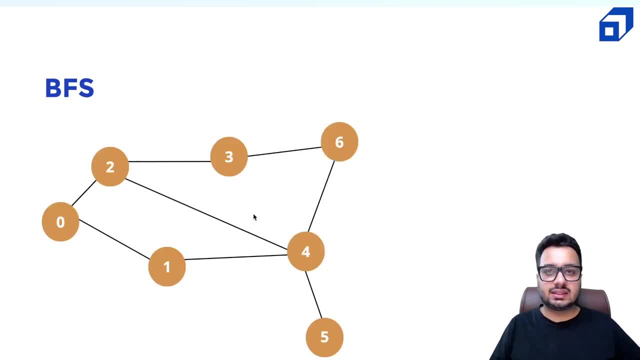 many, many applications, and that is why understanding this algorithm becomes very important. so let us now dive deep into the algorithm. now suppose a graph like this is given. so what kind of graph it is? in my case, it is a unweighted graph, and it is also a undirected graph. that means edges. 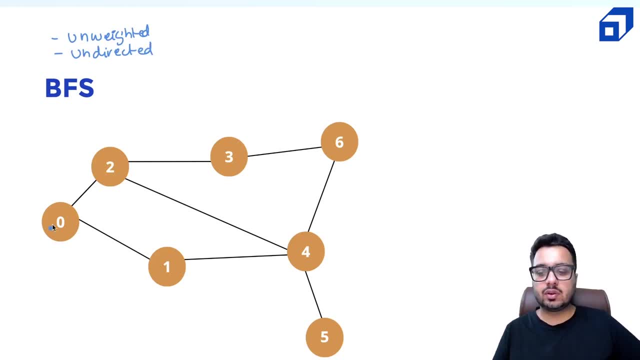 don't have any specific direction. if 0 and 2 are connected, 2 and 0 are also connected, so we can go both sides right. so now in this algorithm, what is the input? the input is a source vertex. that means you are given a starting point. from that point you have to traverse the whole graph. the starting 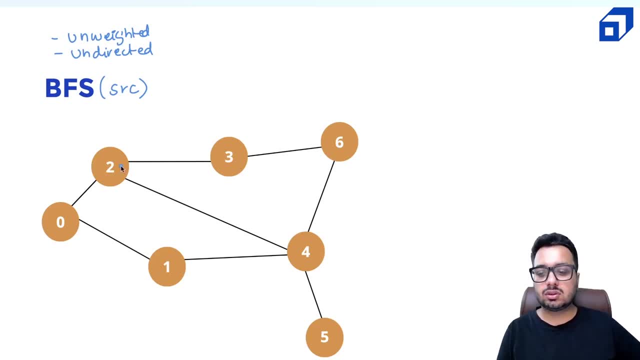 point could be 0, it could be 3, it could be 6, it could be any node. so just to keep things simple, i'm going to take 0 as my starting point, right, and let me also draw the adjacency list that could be possibly a input for this algorithm. so that means 0 is connected with 2 and 1- 1 is connected with. 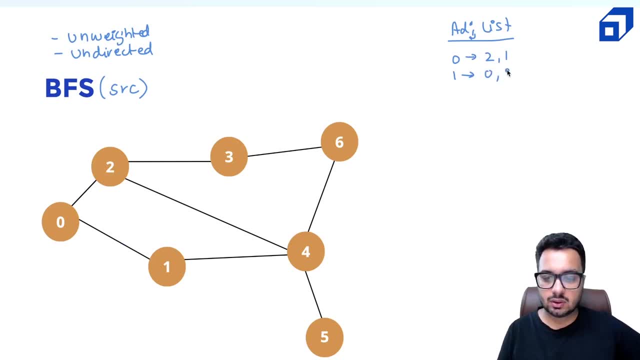 0 and 4. neighbors of 1 are 0 and 4. neighbors of 2 are 0, 3 and 4. so 0, 3 and 4. neighbors of 3: they are 2 and 6. neighbors of 4: they are 1, 6, 5. i'll write it as 1, 5- 6, then i have neighbors of 5. 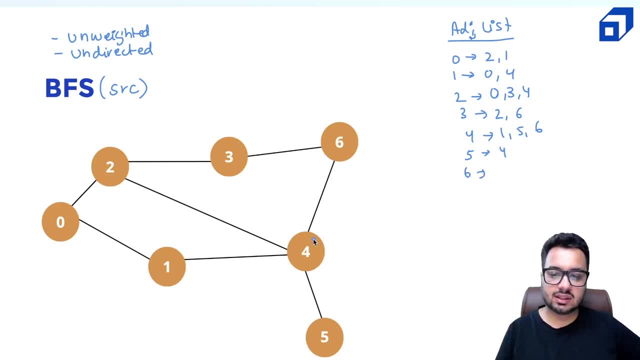 which are only 4, and neighbors of 6, which are 3 and 4. right so far, i have already given the starting point. so this is a node for each node, right? so now let's go ahead and take note of that. one thing: i told you that if you start from this, 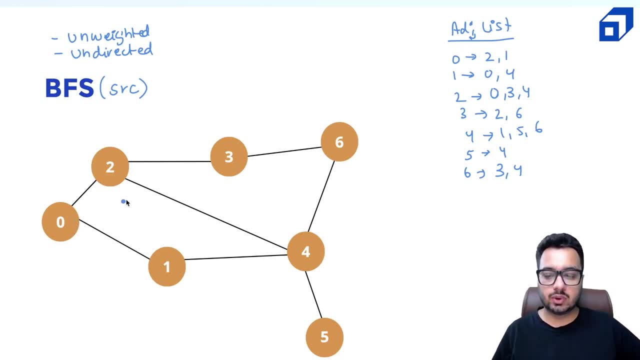 node, right? so what we need to do? we need to. we'll be using a q in this algorithm. you will understand why this q is going to be very, very helpful. let me draw a data structure here which is a q. apart from it, we will also need something to maintain whether a node has been visited or not, right? 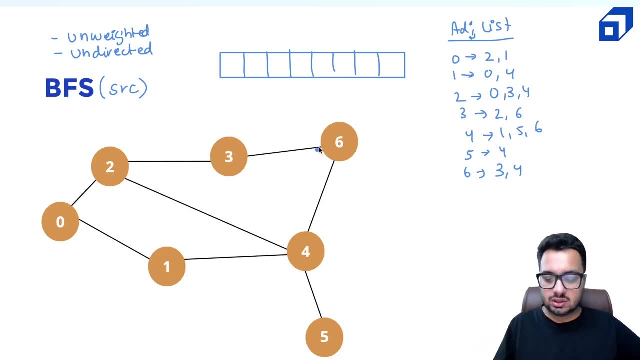 because the graph contains a cycle and it is possible that we are coming to the same node again and again. right, this is a queue. it is a empty queue as of now. right, the queue, you, you know it has a fifo property, first in, first out property, right, so it is a fifo queue here, and apart from it, i'm making one more. 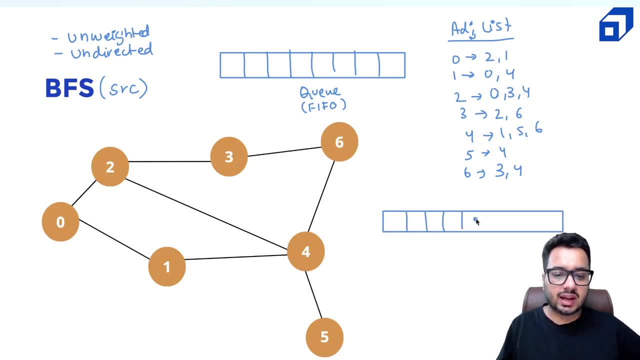 data structure which is going to denote whether a node has been visited or not. so zero, one, two, three, four, five, six. i think this is sufficient. we don't need so. we will mark whether a node is visited or not. so right now it is: nothing is marked, nothing is visited. we'll start from this. 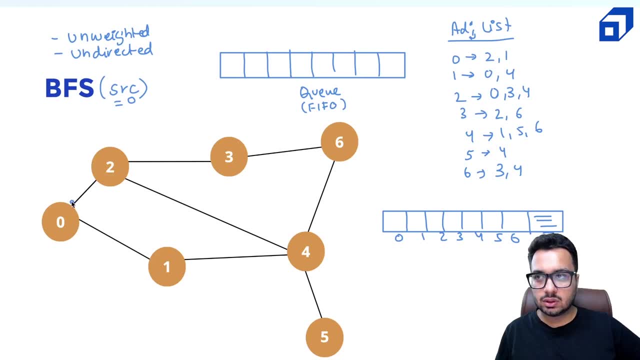 node. that is the source node. let's just assume the source node is zero. we'll mark it and we will put it into the queue. zero has been visited. zero goes into the queue and i am going to mark it as visited. so here the circle denotes the queue has been visited. now, what you will do next? you will look. 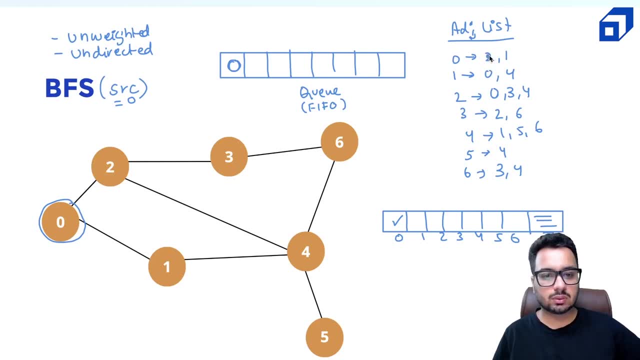 at this adjacency list, you will find out the neighbors of zero. the neighbors of zero are two and one, so you will pop this node out. the node is zero. you will look at neighbors of zero, that is two and one. you will mark them as visited and put put them. put them into the queue. so you from zero, you can easily visit two and you. 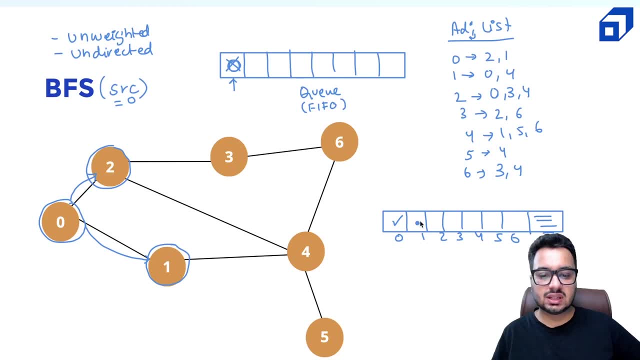 can easily visit one. what i'm trying to do is i'm marking one and two as visited and i'm putting one and two into the queue. so first i visited two and then i visited one- both of them. they are into the queue. that means i have marked one and two as visited. now what you will do next. 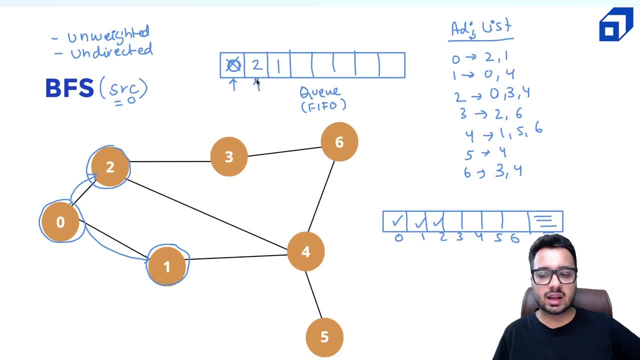 nothing. you simply have to pop out a node from the queue every time and do the same process again. so now you will remove two. look at the neighbors of two, which are zero. three and four. now zero is already visited, so you do not do any work at zero. then three and four. three is not. 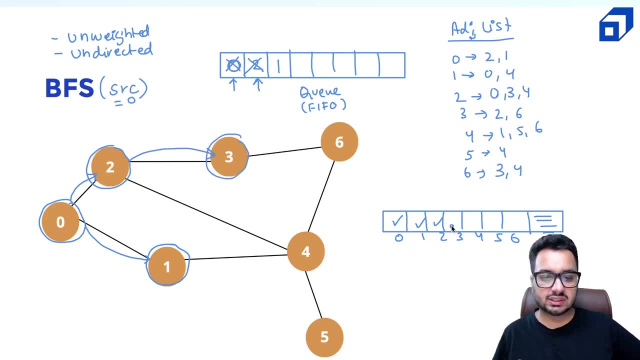 visited. you can visit three. mark three as visited, put it into the queue. and mark four as visited and put it into the queue. okay, now two is gone. two has been removed. next node you will get from the queue, it is going to be one, so you will remove one from the queue and you will mark neighbors of one as visited. so neighbors. 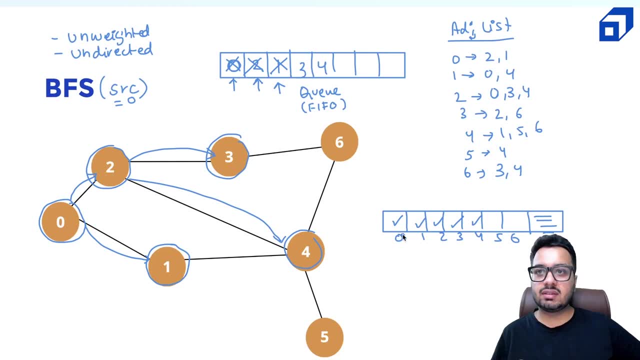 of one, zero and four. look at zero. zero is already visited four. four is also a neighbor. four is already visited. so you do not do any work. so you do not do any work, right? so in the meanwhile, you can do this. two is already visited. so you have seen zero, you have seen two, you have seen one. next you. 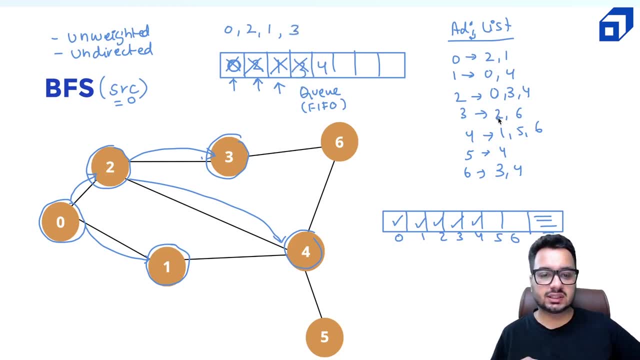 will pop out three. so remove this node. print this node. look at the neighbors: two and six. two is already visited. do nothing at two. six is not visited. to mark six as visit, put it into the queue. so you have to. tre: you have traversed six as well, so six is now also into the queue. next you. 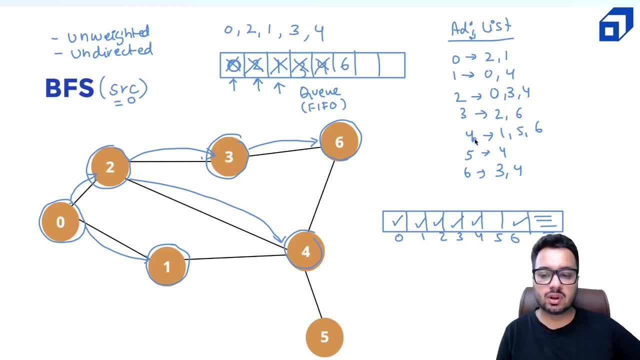 will pop four, So print four. look at neighbors of four. four neighbor is one which is already visited. its neighbor is five, which is not visited. you will visit it. put it into the queue. Six is already visited. do nothing to do here, right? 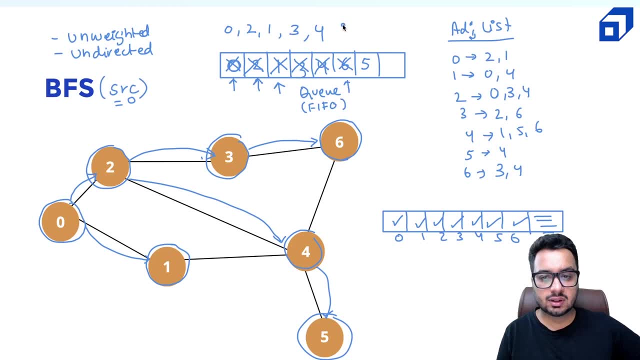 Next you will get six from the queue. remove it and it. and now look at neighbors of six. six neighbor is only three and four right, But both of them they're visited so you will not do any work. So next you will remove five. five neighbor is four. 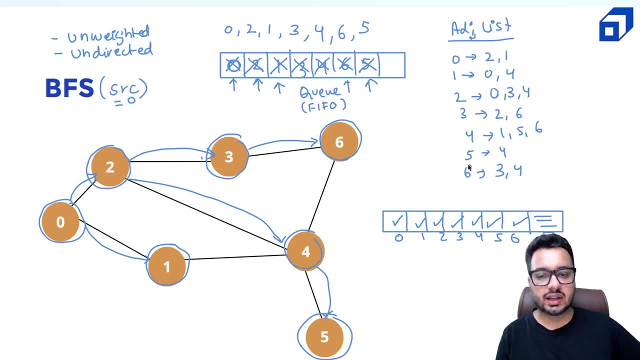 So this is also removed. four is already visited and you do not do any work. And now what you can say is that your traversal is done. right, Your traversal is done. what happened during this traversal? we visited each node once. 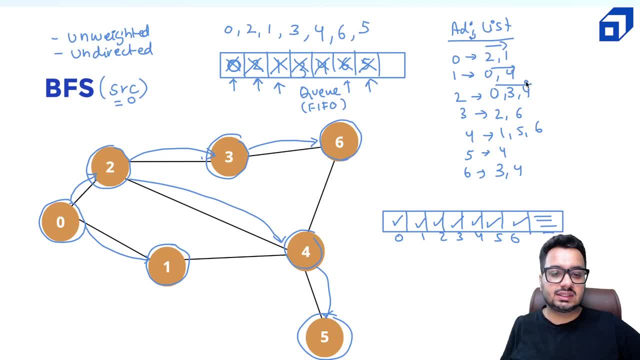 And in the worst case, we are traveling through all edges Once. right what we have done, like we have traveled through, through, through some edges, And we also checked that. from four I can go to one, So we did check this edge right. 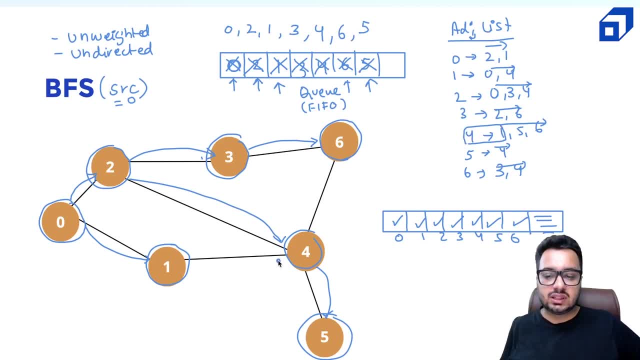 We did check this edge. one was already visited, So we did not mark anything here, right? So we did not mark it in anything. What I'm trying to say is, when you're running this algorithm, each vertex is going into the queue once and it is coming out of the queue once. 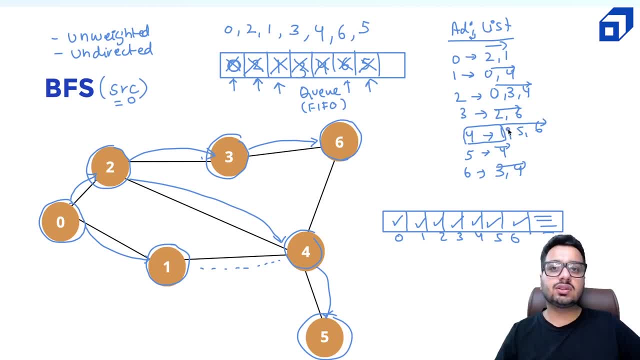 And when you're finding the neighbors of a node, you're traveling through all the nodes right. So all the edges right. All the edges are being covered at most twice. For example, neighbor of four is six, neighbor of six is four. each edge is counted at most. 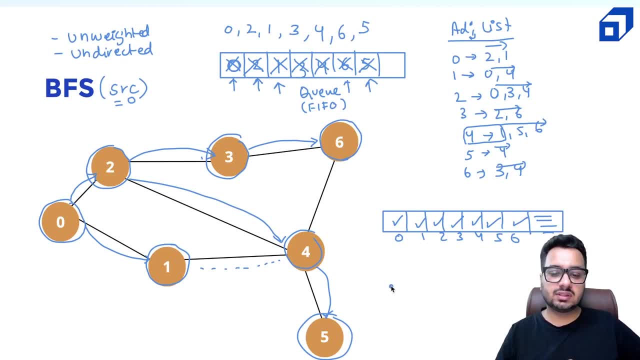 two times. So if I talk about the overall time complexity of this algorithm, it will be linear in terms of number of nodes and number of edges. This is what we are doing, right? I hope you have understood the basic BFS idea. 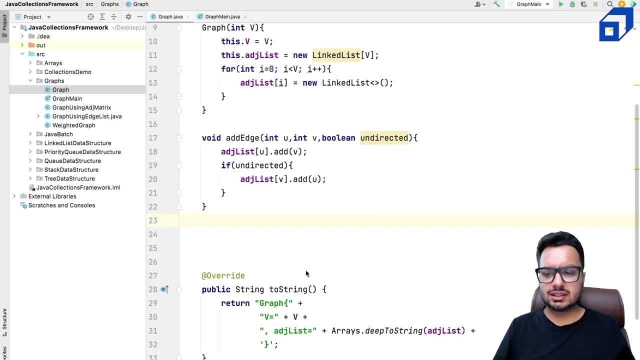 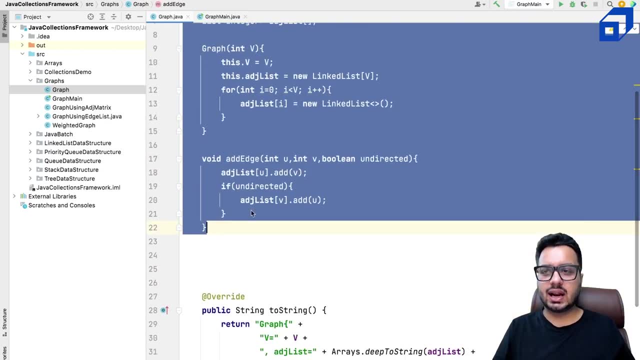 Next we will look at the implementation and code this algorithm. Let us discuss The implementation of BFS. I already have the boiler plate code ready, which is basically adding edges into the graph. The BFS function is something that I'm going to write now. 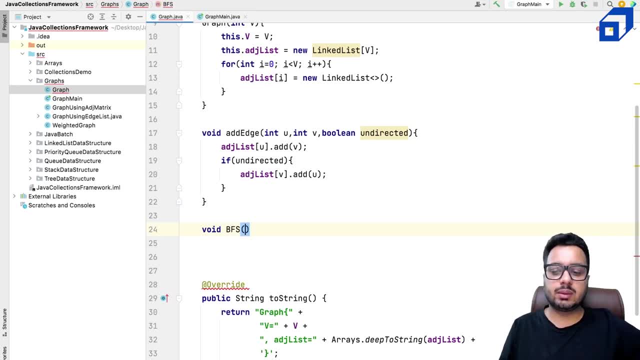 So return type is void. We do not want to return anything. The method name is BFS, but what we may expect as input is one source node from which we should start doing the BFS for this graph. So this is the graph. So I told you we will be needing two data structures. 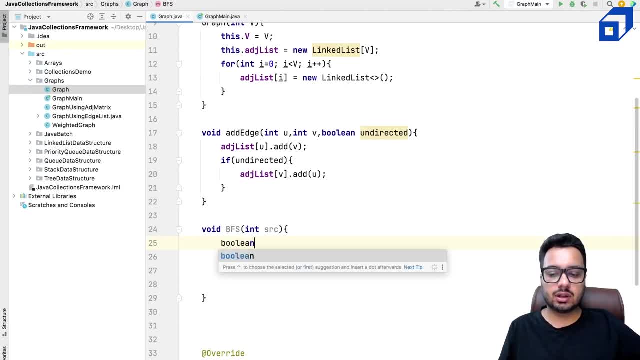 One to maintain Whether a node has been visited or not. I can maintain a Boolean visited array, And this will be an array of size V, where V is the number of vertices in the graph. Next thing I will need would be a data structure Q. 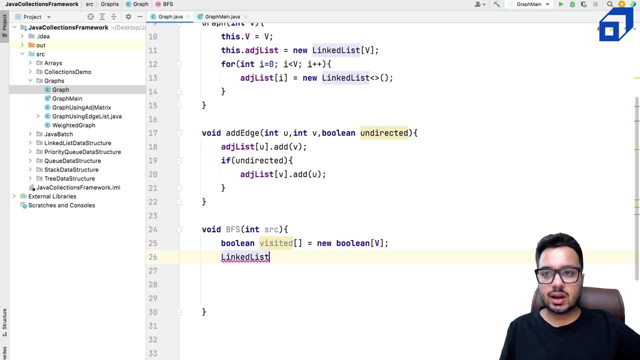 So in Java we have Q as our interface. I will create a linked list which provides me with the implementation of Q as well: Linked list of integers. We will just call it as Q and I will say this is equal to new linked list. 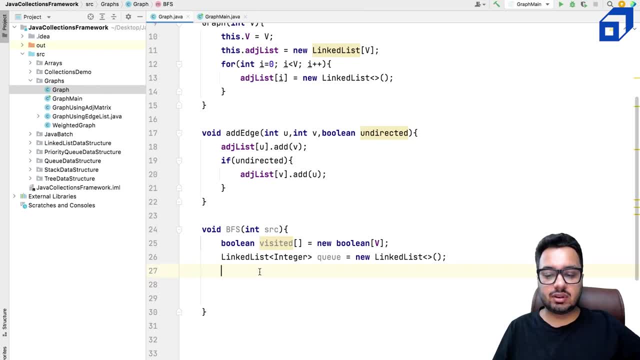 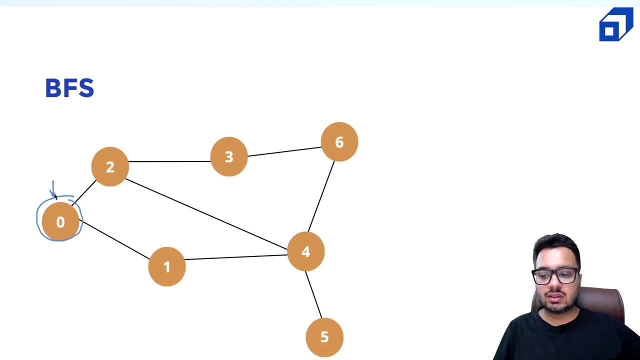 All right, so that are the data. These are the data structures that we will be needing. Let's start with the algorithm In the first step. what I will do? I will start with the source node: market as visited. push it into the queue. 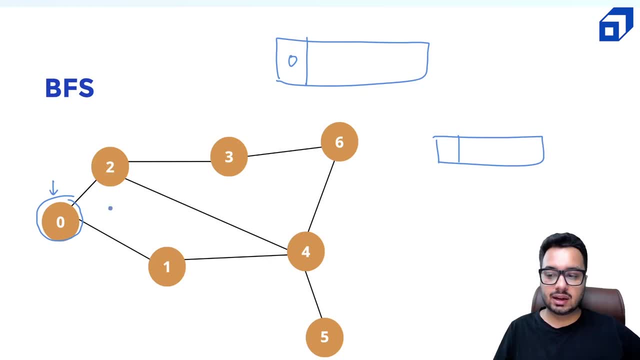 So I have to do three things: Market as visited. So visited of source is going to be true. Okay, This is going to be true. And then I will traverse the neighbors of this node. So first thing I will do is I will push this into the queue. 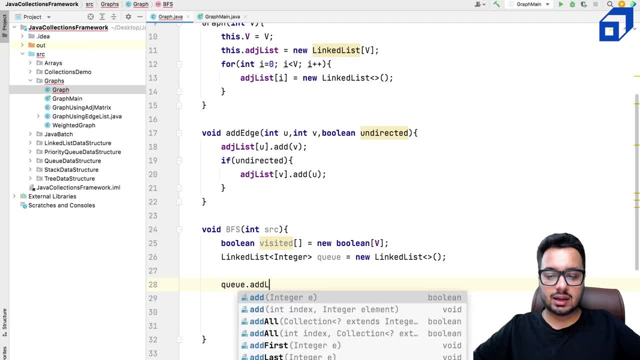 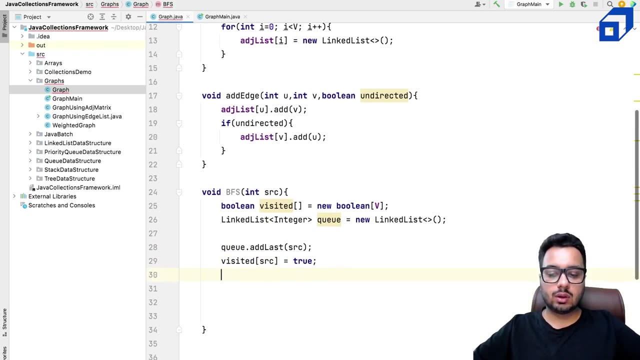 So I can say your dot add last. the node is source. okay, And second thing I will do is I will mark this as visited, visited of source. this is going to be. what can I do now? I can do while my queue is not empty. 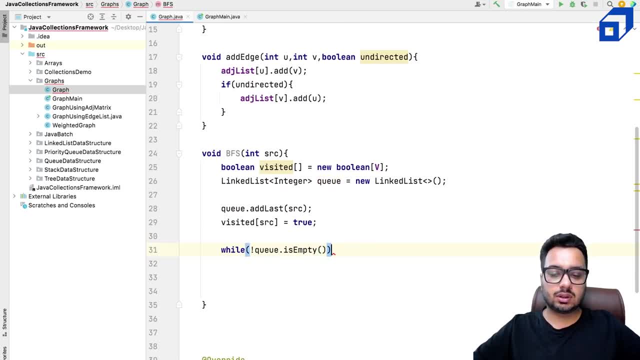 So I will stop once all the nodes have been popped out. So how do I add into the queue and remove from the queue? You know, if you have to add something into the queue, that addition will happen from the ending. So add last. 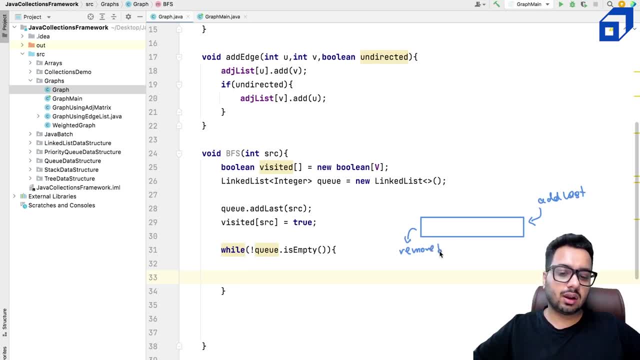 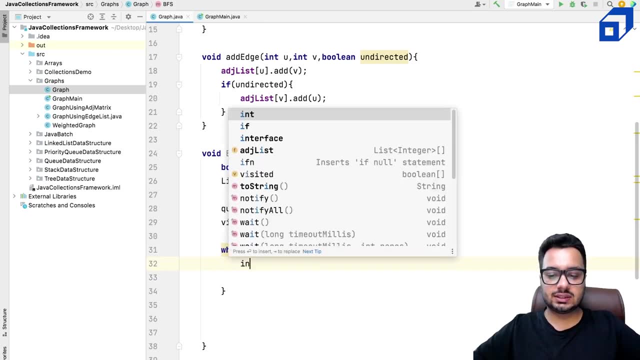 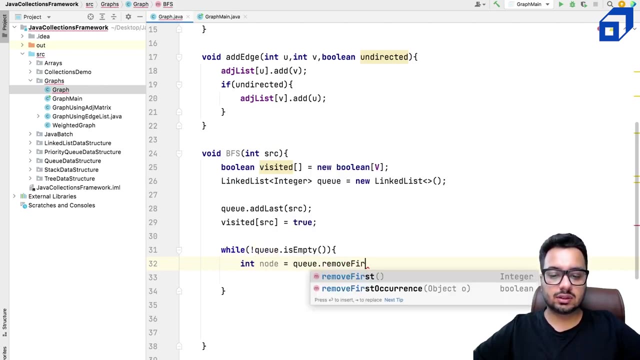 And if you have to remove something from the beginning, we can call remove first method back into okay, the node at the front of the queue. So that is int node. This is going to be queue Okay. Okay. So I am going to remove from the queue dot. remove first. 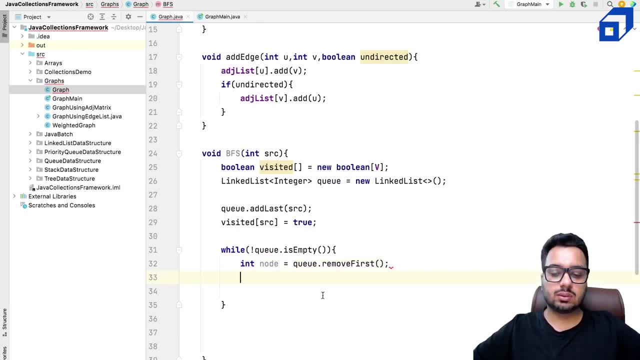 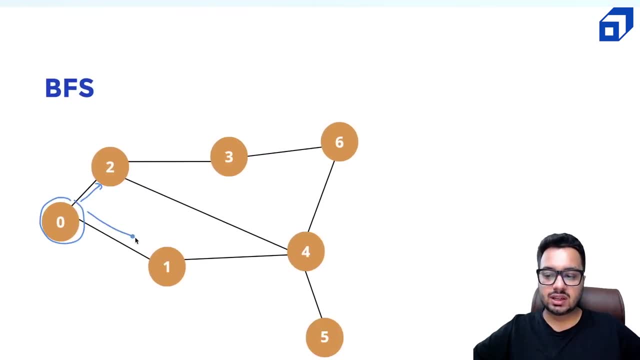 All right now what can I do? I can say okay for this node, so node that I've removed from the queue is zero right. So I need to traverse. what are the neighbors of zero? zero's neighbors are there in adjacency. 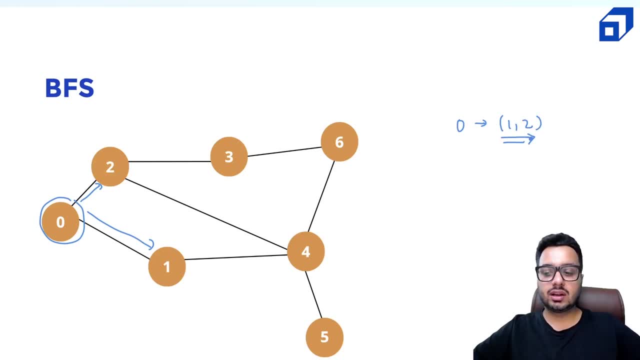 list. So they are one and two. So what I need to do, I need to traverse on these neighbors. If the neighbors are not visited, I will mark them as visited and I will push them into the queue. So this is what I do. 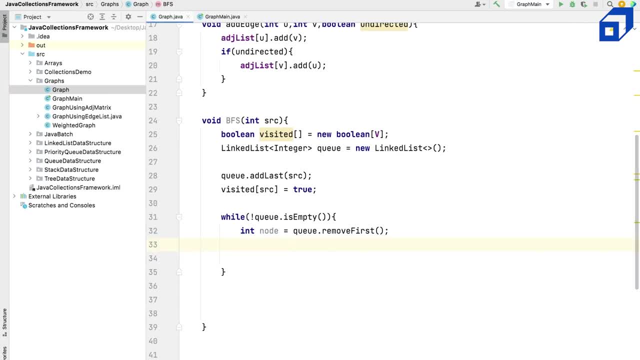 I can say, okay, for every neighbor. okay, so to get the neighbors what we can do, we can use iterator. I can create a iterator of the type integer and call it something like iterate it, and now I can say: give me the neighbors of this particular node. 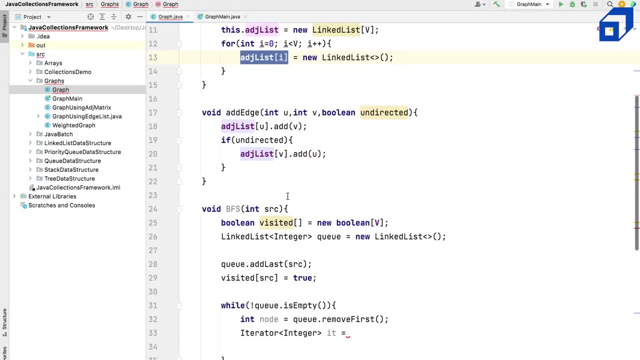 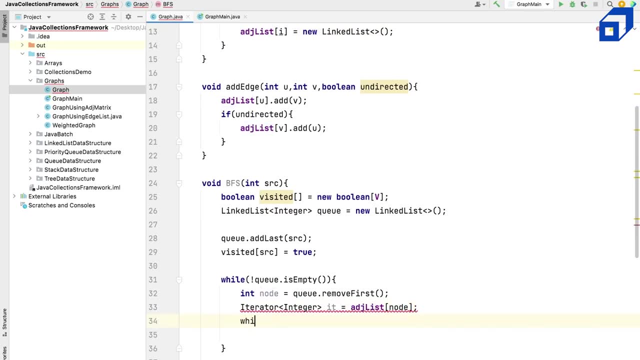 So if you know, then this is the adjacency list type. I want to iterate on this adjacency list So I can say, okay, while it dot has next, that means the next node is present. basically it is a way to iterate on the adjacency list or you have to call a method called list iterator. 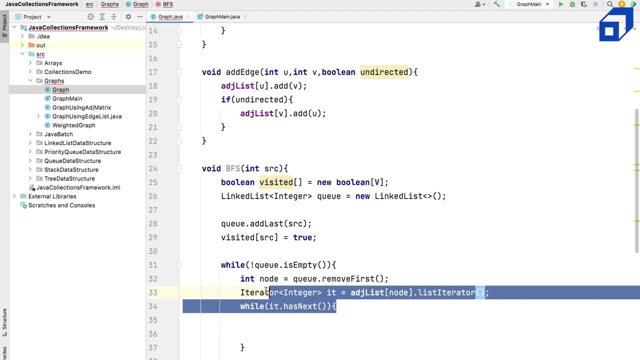 because we are iterating on the linked list. So zeros, zeros, neighbors are one and two, right. These are stored in a list, which is which was a list object, So adjacency list of nodes. Okay, So the next node is a list. we have to get the iterator using this method: list iterator. 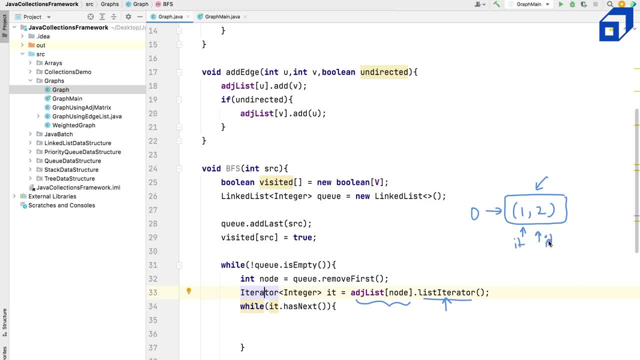 So it will iterate over these nodes until the list is not finished. it will go over these neighbors. Now I want to get the node right. So how do I get the node? I can do. okay, the neighboring node is nothing, but it dot next. 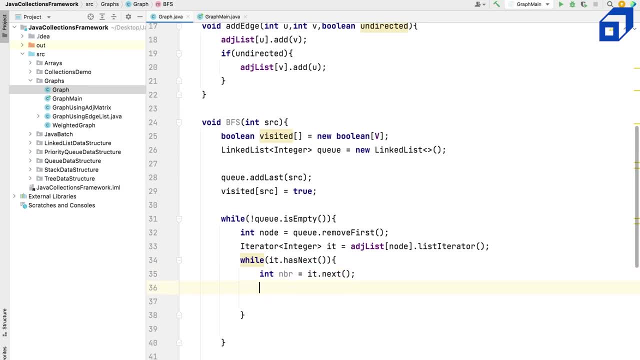 that is the neighboring node. And now what I need to do. If it is not visited, if not visited neighbor, what do I need to do? I need to mark it as visited. I can say visited of neighbor. this is equal to true and I need to add it into. 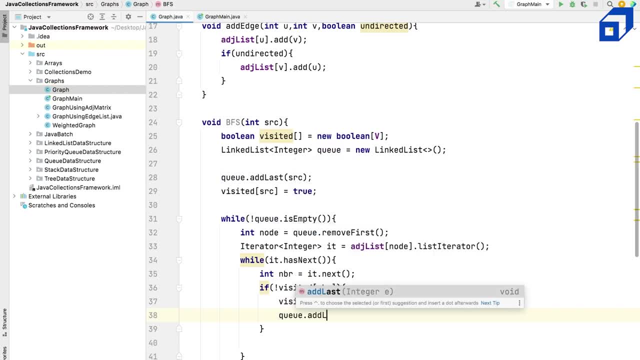 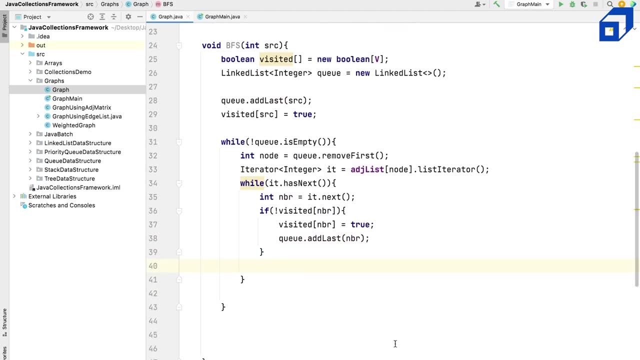 the queue. So I can say q, dot and last, and the item is neighbor, we are iterating over all the neighbors And if the neighbor is not visited, we simply mark it as visited and we push it into the queue. I hope this should suffice. 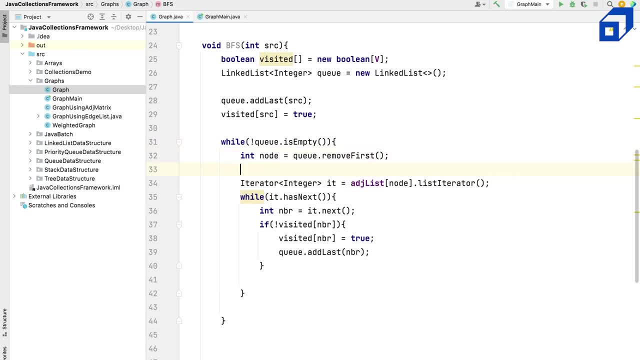 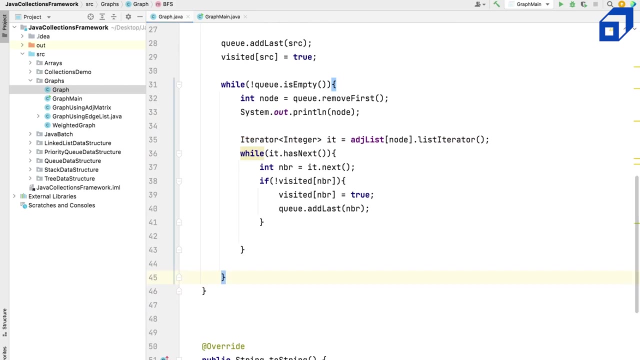 And one more thing we can do: in the while loopers we can print out the node. we can see what output do we really get? I can say: s out node. Now let us test our algorithm on the graph I have already constructed. 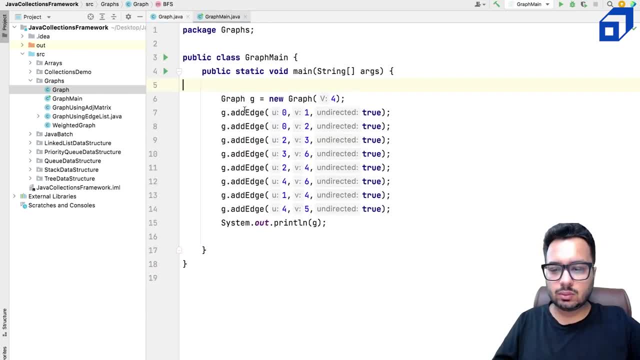 So let me show you in graph main. I will go, And this is the graph, Same as this graph, And now we are going to run BFS function on it. I can say g dot, BFS. let's say the source node is zero. 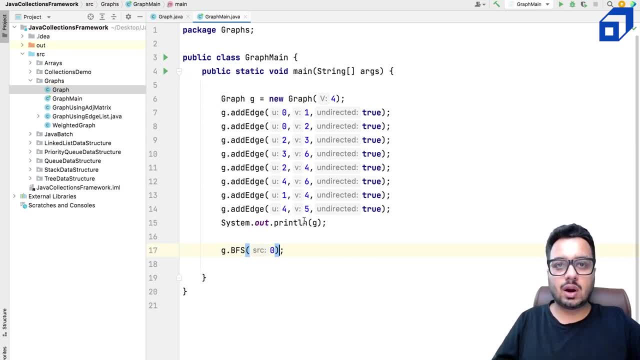 So let's go and run this code and see what output do we get. We should get all the nodes from zero to six, because we are doing a graph traversal. Let's see the output. Okay, we got an error index six out of bounds for an error. 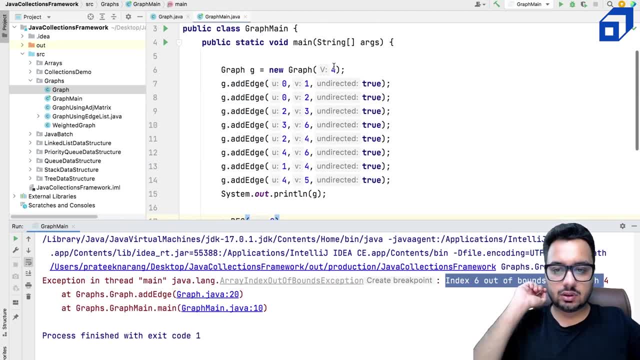 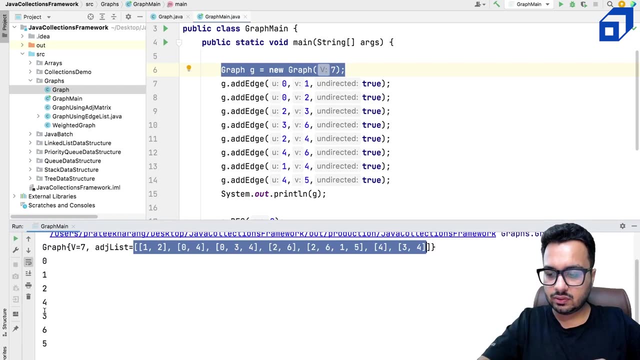 So let's see the output. Okay, We got an error of length four. Okay, so here we have to give. we have seven nodes actually. input needs to be fixed. Okay, so this is our adjacency list And we are getting 014365. we are getting all the nodes. that means the graph traversal is: 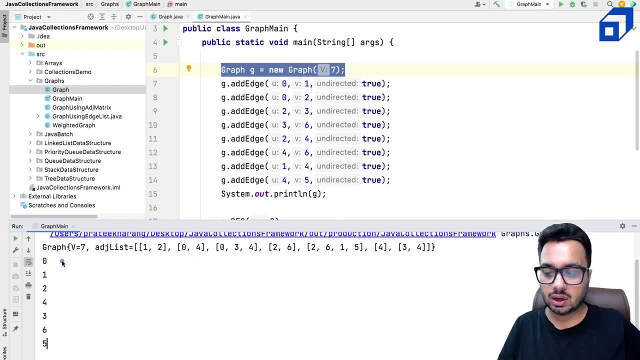 correct. Now the exact output will also depend upon the way you have stored these nodes, Okay. So you said: okay, zeros, neighbors are one and two. After zero it will print one and then two. But if you say in my adjacency list I will store two and one first. 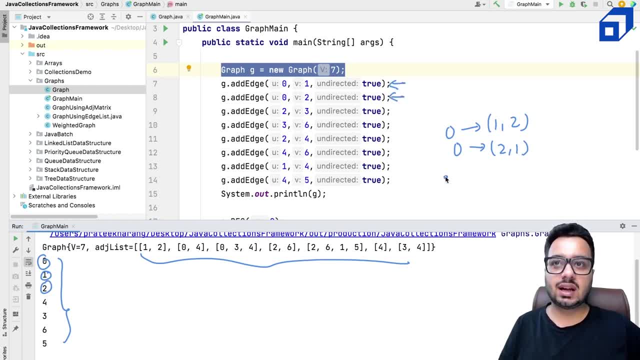 That means I will add this edge before this edge, then the output will be zero to one, and so on. Right now, our goal was to visit all the nodes which are which can be reached from node zero. So we are getting 012436 and five. 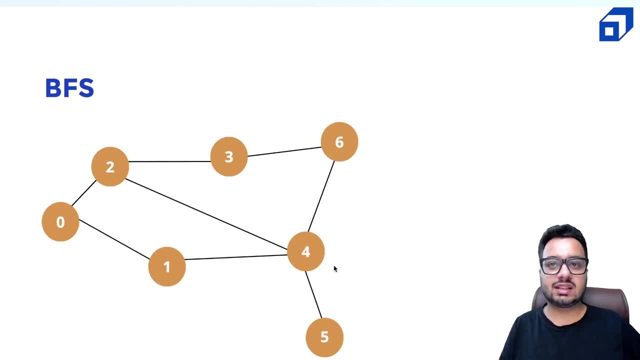 That means this output is correct. we are able to reach all the seven nodes, Including zero. Now let us discuss one application of finding the shortest path from the source node to all other nodes. Okay, so what we are going to do, we're going to do shortest path from source to all other. 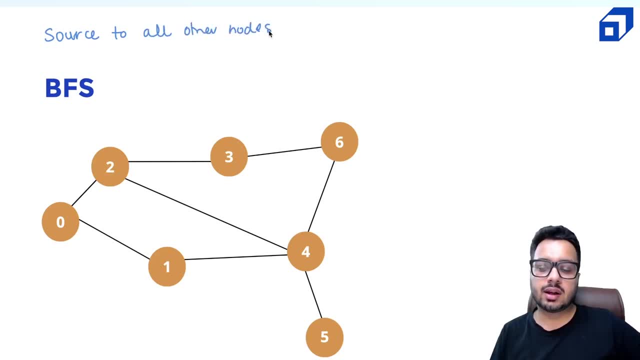 nodes in an undirected graph, in an unweighted graph, unweighted graph. So this graph is an example of an unweighted graph. So graph can be directed or undirected, But it must be an unweighted graph for the BFS algorithm to work for finding the shortest. 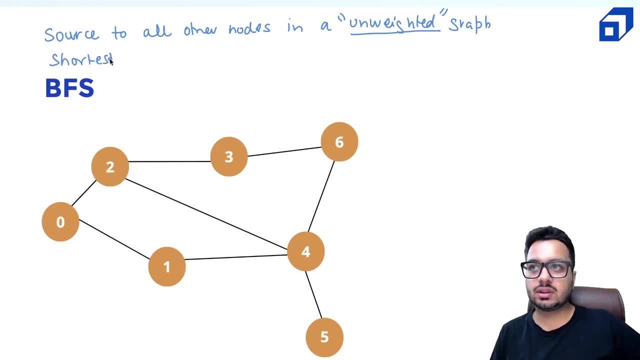 path. So we are going to talk about BFS- shortest path algorithm. The algorithm is very simple And it is very similar to just doing BFS. Let us try to visualize what we are doing. in BFS, We are starting from node zero And we can mark the distance of zero as zero. 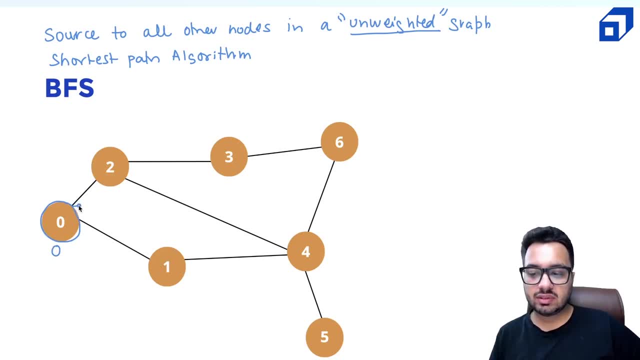 And from zero we are visiting the nodes one and two. Since we are visiting a node for the first time, we will be updating their distance And we will be saying: this distance is one And this distance is also one, because we are coming from zero and zero distance is zero. 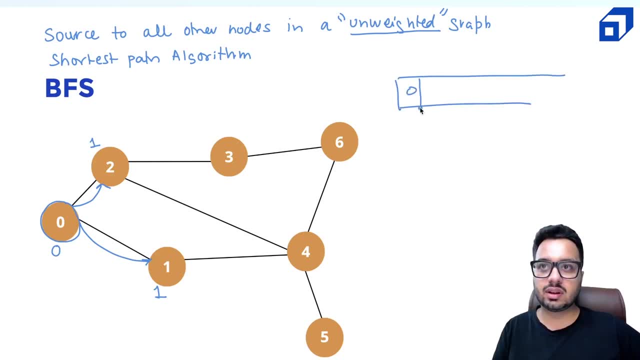 Next. you know in the queue what you have done. you have said: okay, zero is there. then you pushed one, and you pushed two, and so on it Now next. next item you will pick is one and you will update the neighbors of one neighbors. 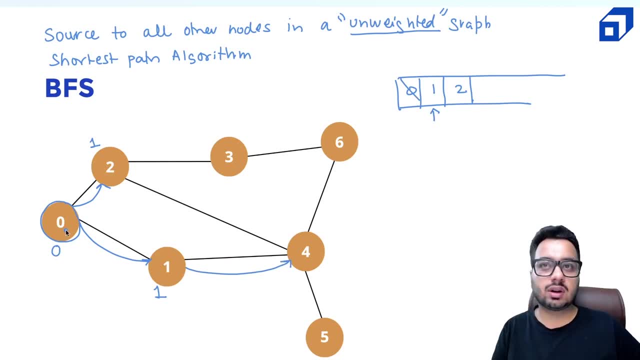 of one is it's a four And zero Zero is already visited, So you will not go there. So you will say: okay, since I'm visiting for via one, this distance must be to the distance of four. I can say distance of the neighbor is one more than the distance of the parent. 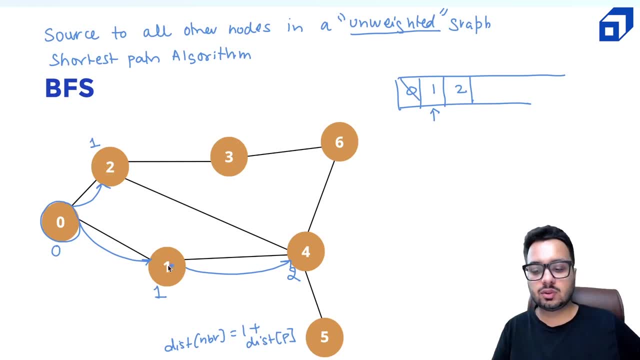 to parent is one. okay, distance of parent, parent node is one, child node is four, or the neighbor node is four. four distance is one more than the parent. I will visit four and I will push four into the parent, Okay. 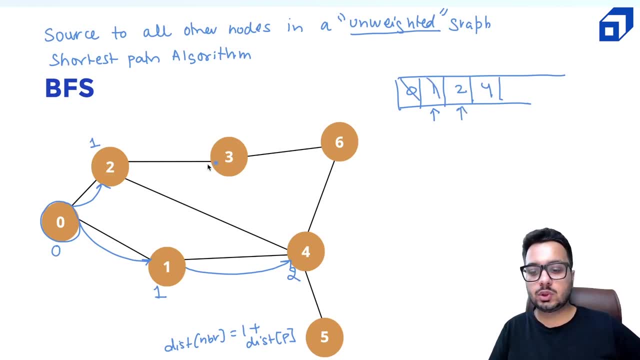 into the queue. Next I will remove two. two neighbors are zero, already visited. three, three is not visited, So I can visit three And I can. okay, this distance is going to be two, So I will push three into the queue. 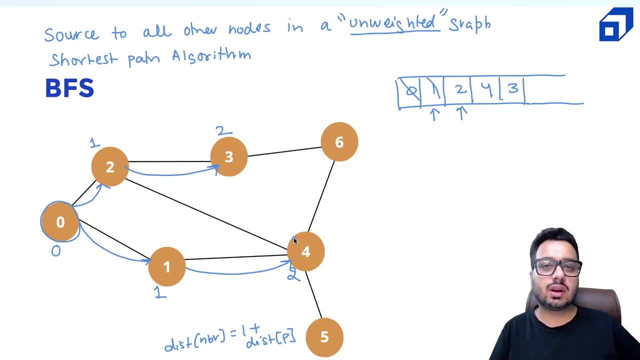 And two neighbors is also four, but four is already visited So we will not update it. but it is not possible that you're reaching a node later which is already visited and the distance will get minimum. it's not possible in case of an unweighted. 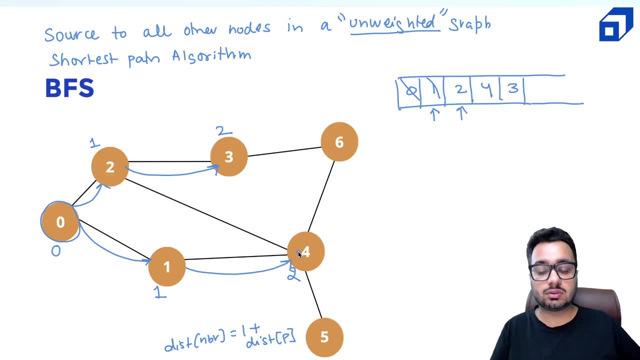 graph if it would have been weighted graph. this was, this could have been possible right Now. four is already visited And since you are reaching from two, again node is already visited, So this distance will be either greater or equal to two. so it is, we will not update. 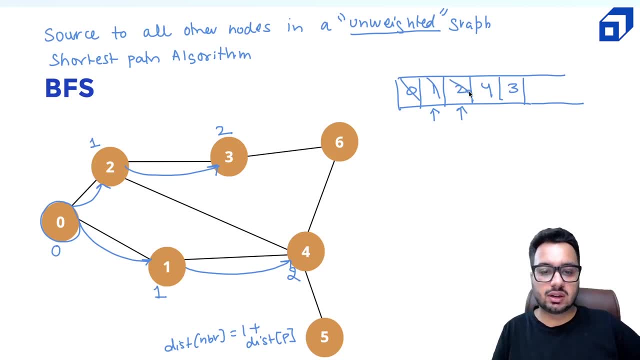 it. So we will not do anything at four. So two is done. two has done its work. Next we'll pop out four, and four can now update its children. So four children are six. This does not work. Okay, This distance is three. you push six and four can also update five. this distance is: 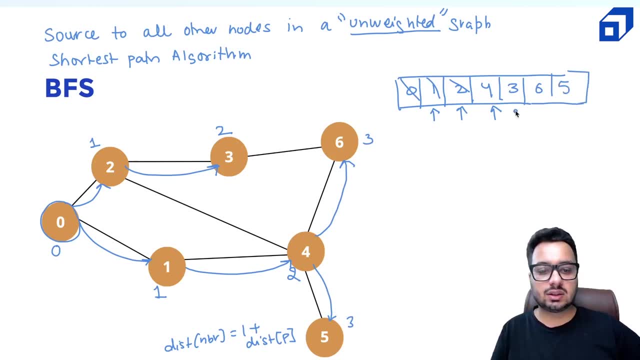 also, you can push five. Next you can pop out three or three again. it will try to visit six, but six is already visited. So hence you don't do any work And you try to pop out six. you can remove six easily. 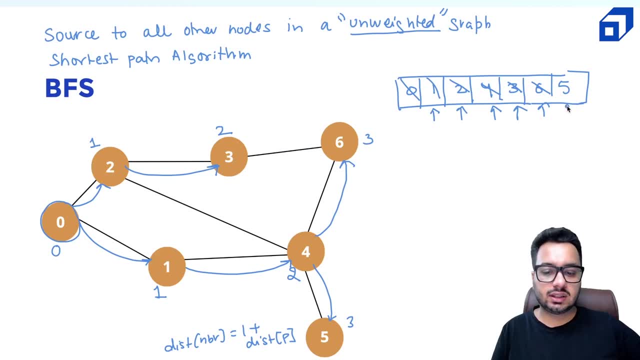 But there are no nodes or neighbors of six which are not visited And you pop out five. there are no neighbors of five which are not. So if you look at these values, you will find that these are the shortest distances from zero to all these nodes. 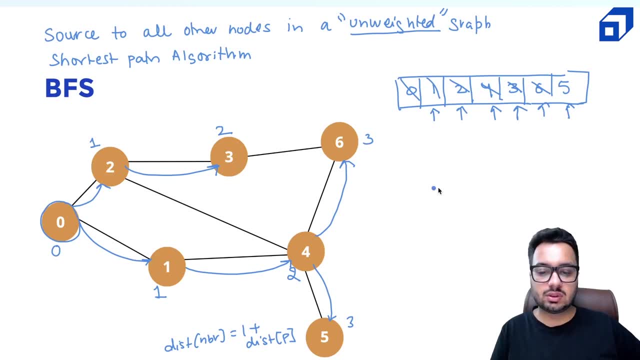 These are the shortest distances from zero to all these nodes. That means distance of zero is zero, distance of one is one, distance of two is one, distance of three is two, distance of four is two, distance of five it is three. and distance. 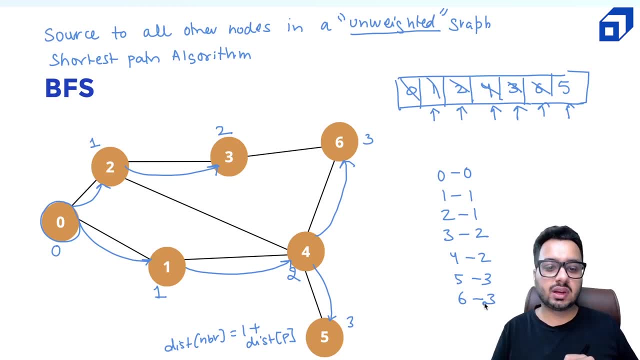 of six, it is three. So one observation we can make out from here is That BFS visits nodes in increasing order of their distance from the source node. This distance was zero, These two distances were one, these two distances were two and these two distances were three. 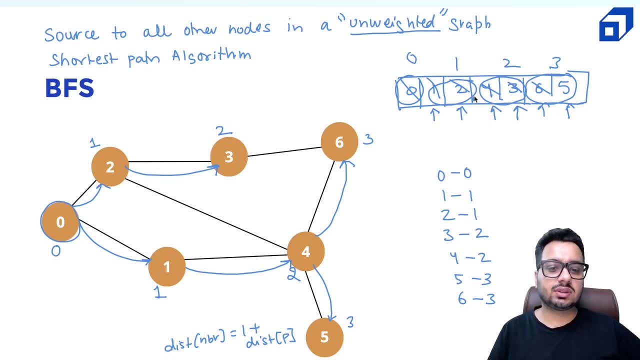 This is an observation. So when I said you can get any ordering, so that means between these distances the ordering can change. So BFS might produce an output like zero to one, it might produce four, three, it might produce three, four, five, six might get five, six or six, five, right. 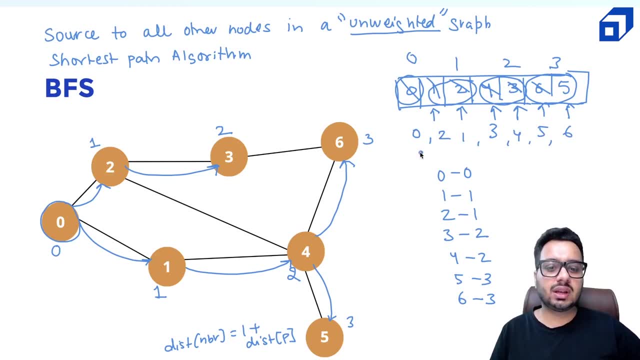 Different orders, But the distances of these nodes will be in increasing order from the source node. That is how we can find shortest path from source to all other nodes in a unweighted graph: by simply using the BFS. In the next part we'll show you the code changes that we need to do for this algorithm. 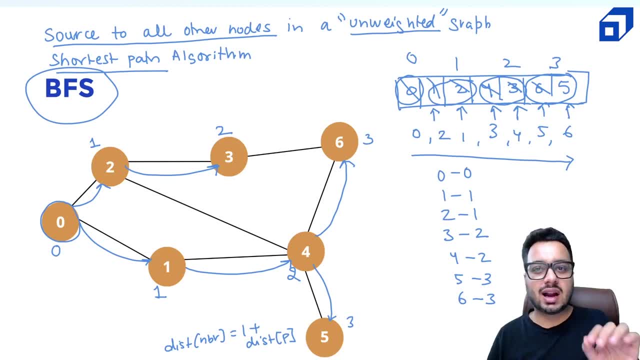 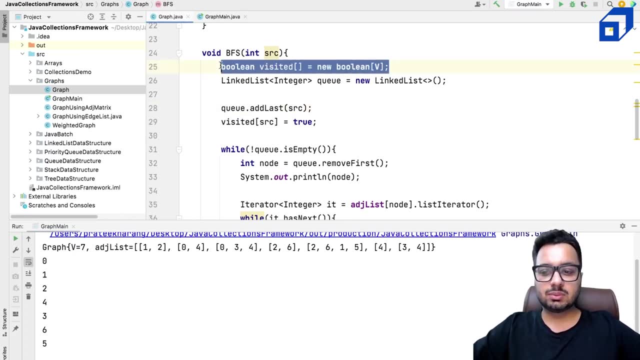 So it is very simple: Take a moment, pause the video And think what changes you will make into the code. Alright, so let us discuss the code changes Now. apart from the visited array, what do you need to do? you need to maintain a distance. 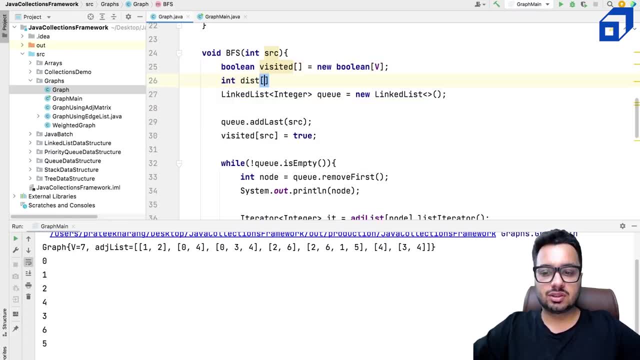 array the distance of each node from the source node. you can do okay. I need a distance array which is of size v And in the beginning you can say distance of source. you can update that distance of source as zero. 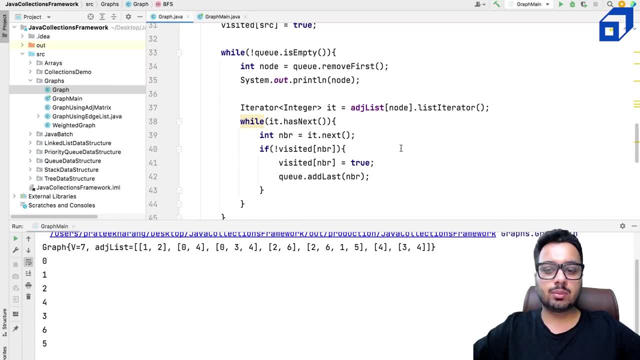 And rest is very simple. As your visiting more and more nodes, you need to update the distance you can do. okay, I'm going to visit the neighboring node, So when I'm visiting this neighboring node I can say distance of this neighboring node. 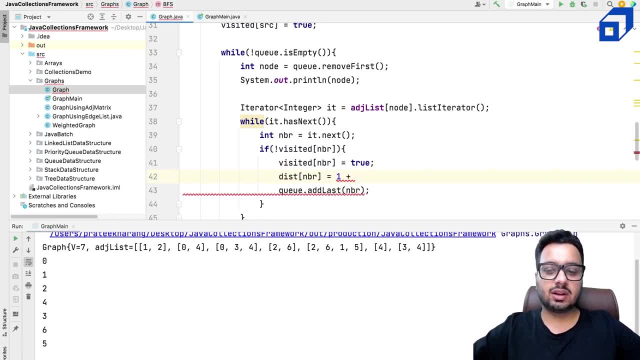 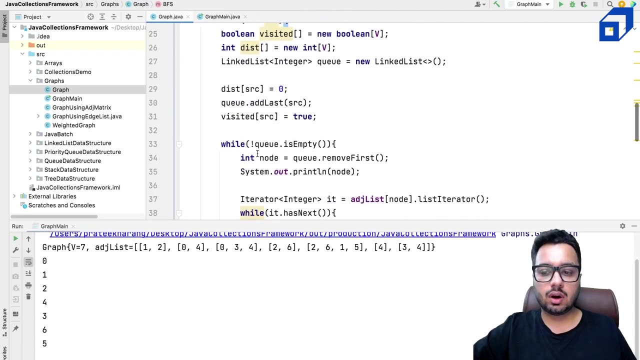 is one more than the distance of the node that is parent of this node. that node is nothing but this node. So this node is distance of node. So that's it Now what we can do in the same function. maybe we can either return the distance array or 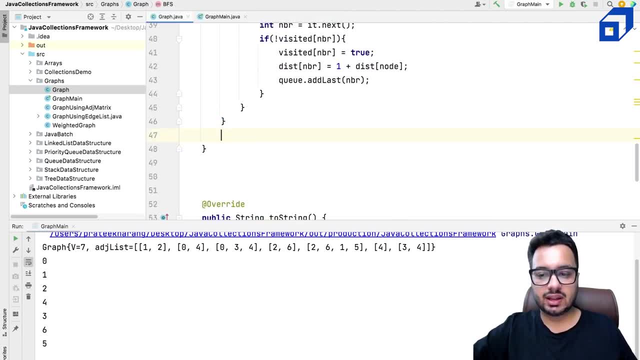 we can just print the distance array. So here I can say: let's just iterate over the distance array. or I equal to zero, I less than v, I plus plus. I can show the node which is going to be I, followed by the 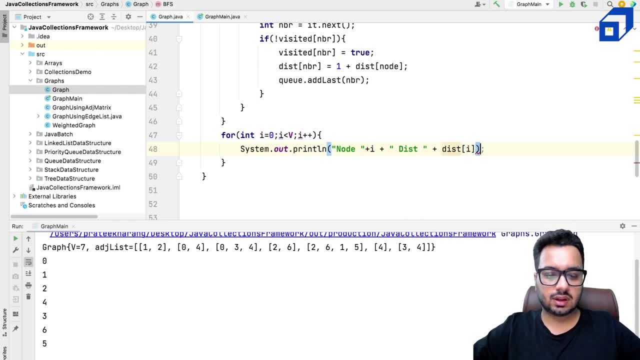 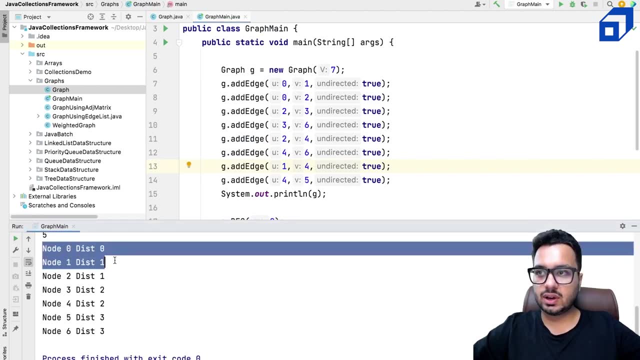 distance, which is distance of I. let's go and run this code And we should see We're getting node zero at distance zero. one at one, two at one, three at two, four at two, five and six. they're at distance three. 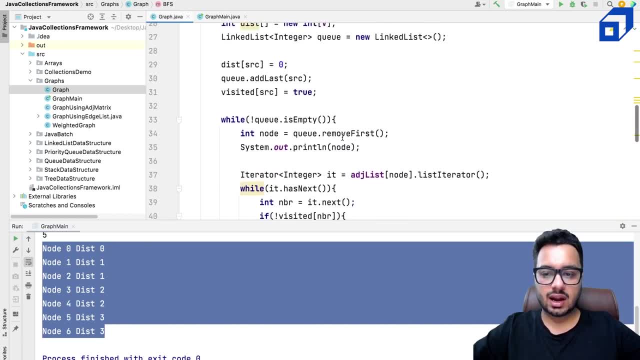 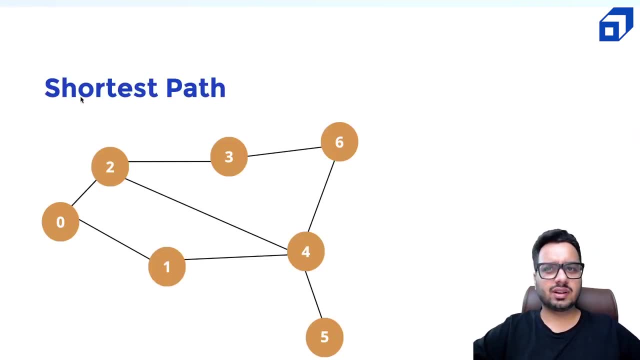 This is how easy it is to make changes in the code. And now we have made shortest path algorithm using BFS. Some of you might be wondering that, okay, we have figured out the shortest path, but we have only figured out the distance. actually, what if I actually want to figure out the 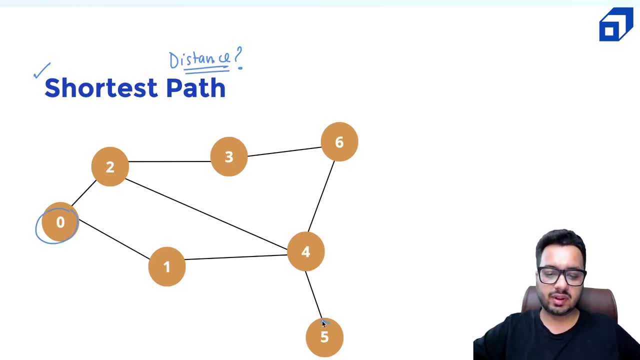 exact path from, let's say, zero to some node five Maybe. I want to find out what is the shortest path. should I go like this, Or should I go like this, Or should I go like this? What will be the shortest path from source to destination in a unweighted graph? 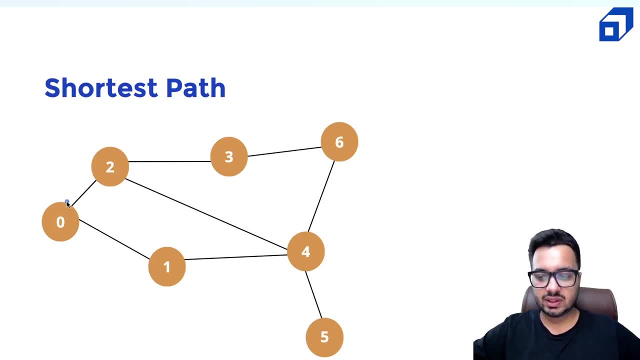 So again, this thing is very simple. What we were doing, we were doing BFS. zero was visiting one and two, one was visiting four, two was visiting three And three was visiting Six. No, I think it was like this: or was visiting five and six and then three, something like. 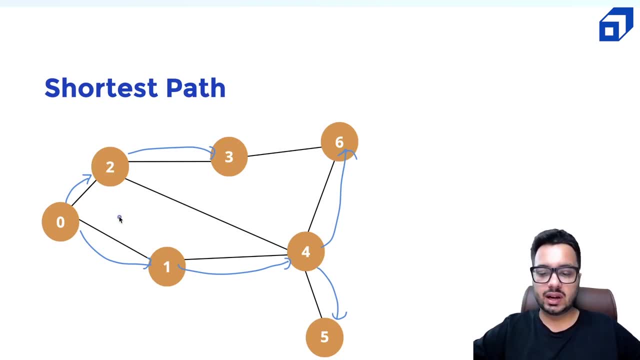 this with it right now. again, if you want to find out the shortest path to reach five, you will know that, okay, five was visited from four or was visited from one and one was visited from zero. right, What you can get, you can. you can actually store the parent so you can store parent of. 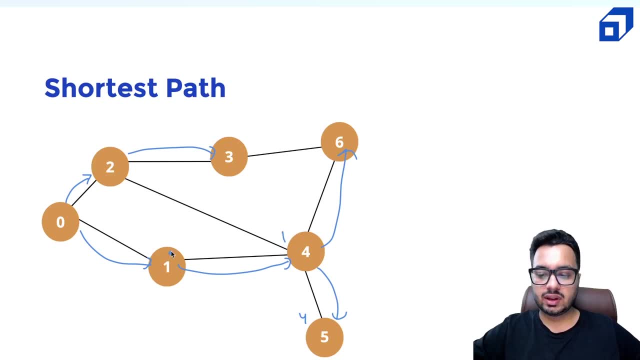 five is for parent of four is one, Parent of one is zero and parent of zero is, let's say, zero or minus one and anything you can put, what you can do, you can store these parents for every node And then you can do trace back. and okay, I'll start from five. 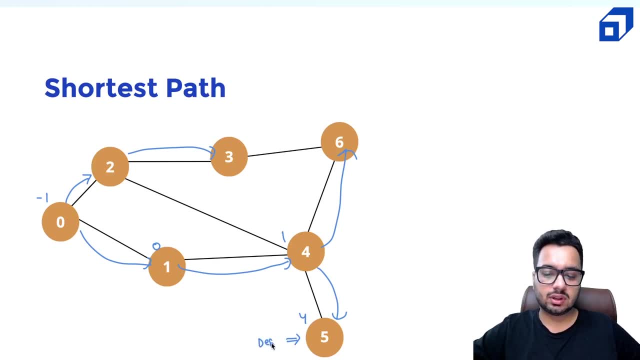 And, okay, from where I should go. This is my destination node. who is the parent of five? how do we arrive at five? we came from four, So I can go to this node. Okay, how do I came at four? I came from one, so I can go to this node. how do I came at? 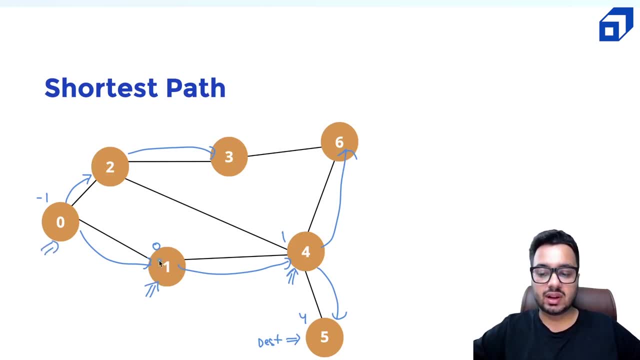 zero, I will go to zero. Okay, how do I? came at one, I came from zero, so I go to zero. who is the parent of zero minus one? That means we have finished the entire path. In this way, you will be able to store 5410 in an array or in an array list. 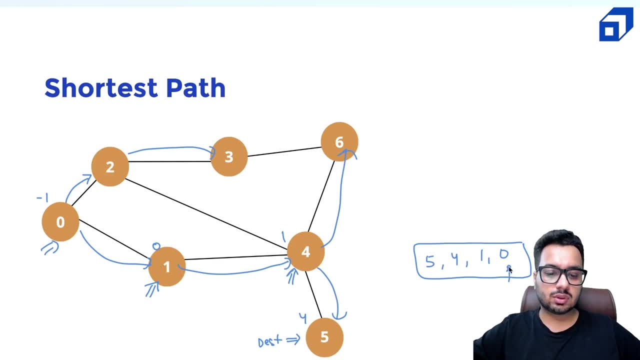 This way, you can also print the shortest path from the source node to the destination node. The only changes in the code you need to make is you need to create a parent array, And when you're visiting from a node to destination node, you need to create a parent array. 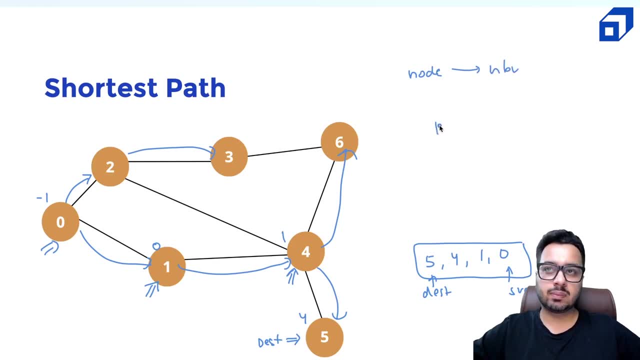 And when you're visiting from a node to destination node, you need to create a parent array To a neighboring node. so you can do: okay, parent of neighbor will be equal to node, something like this, And then you can simply put a while loop at the end. 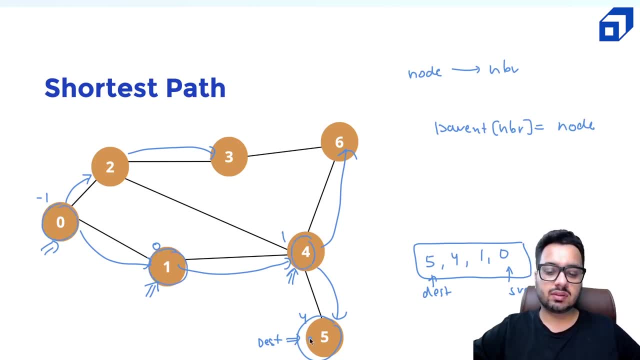 Once all the nodes have been updated, your BFS has been done and okay, while I don't get the source node, let me travel back from the destination node. so you will travel this way, You will travel this one, you will eventually reach the those. 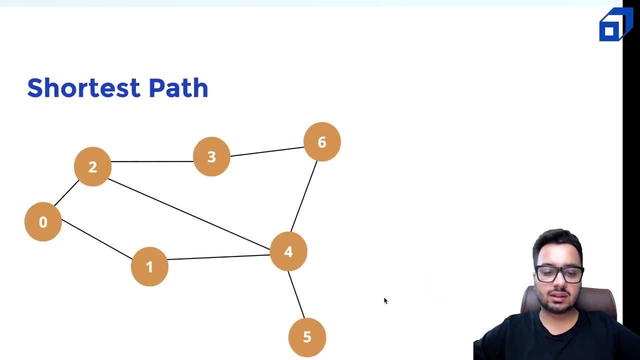 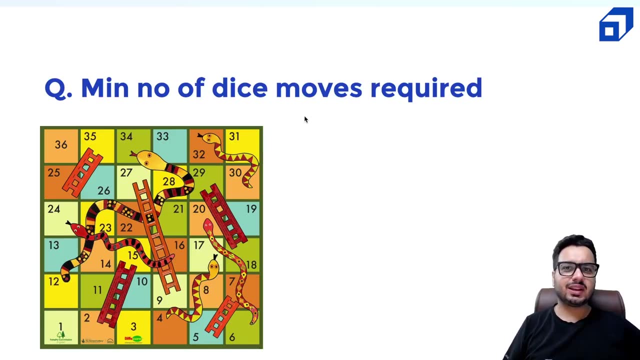 So this is something you have to try, you have to figure out, you have to make the required changes in the algorithm that we have discussed. now we will discuss one application of bfs in solving a problem. so we are given a snakes and letters board which looks like this, and what we 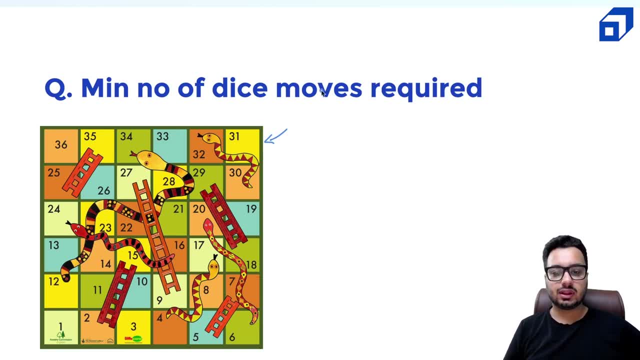 need to do is we need to find out the minimum number of moves that are required to go from source, which is from cell 1, to destination, which is cell number 36. so first of all, we need to decide whether it is a graph problem. so if you look carefully, you can analyze that. we can clearly. 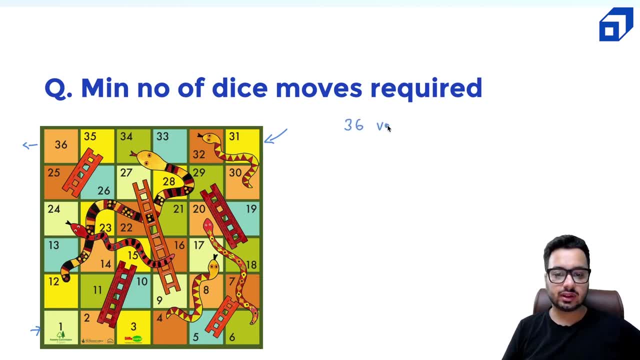 see there are 36 vertices, there are 36 nodes where you can go. so clearly we see vertices, but how do we decide the edges, right? basically it? the question says there is a regular dice, so on your dice you can throw any number of your choice from 1, 2, 3, 4, 5, 6. right? so the rules of the board are. 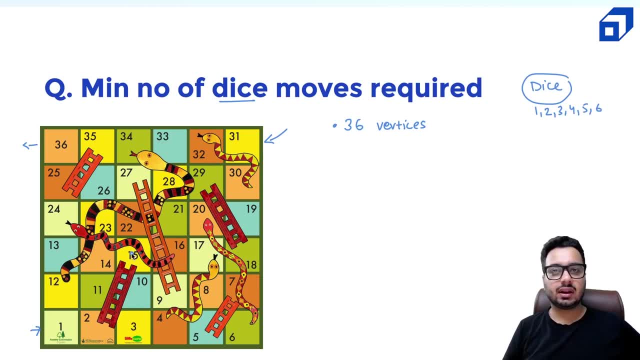 very simple: whenever there is a letter, you can client that ladder, but whenever there is a snake, you will be cut by the snake and you will reach the tail of the snake. so you can cut down from head of the snake and you can reach the tail. this position. 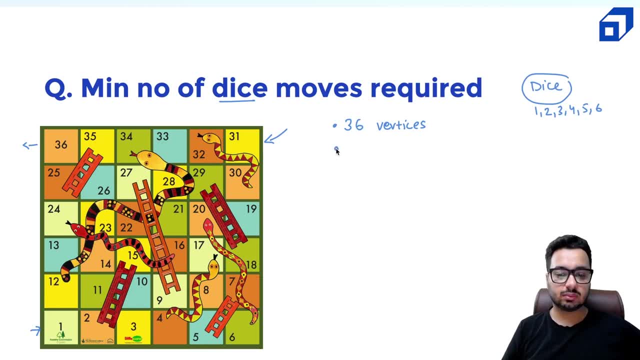 right. basically, like in any snakes and let us go, you have snakes which can cut you down and bring, bring you down, and there are ladders which you can climb and move to the top. the question is how many minimum number of dice moves will be required to reach this destination? so you can assume there is. 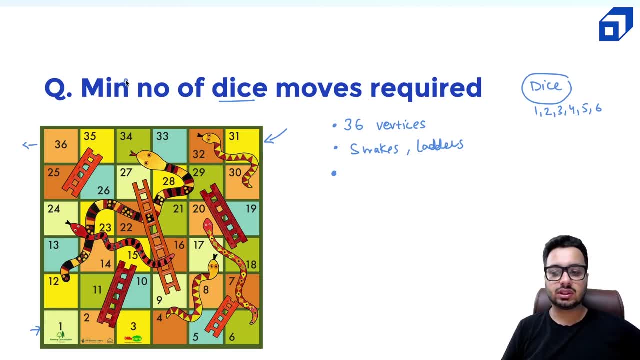 only one player. it's not a two player game. so the question is only about finding the minimum number of dice. now we need to think carefully what kind of graph it is. if you analyze carefully, you will analyze that. if we count the, if you look at the dice moves so at one you can throw a one. that means 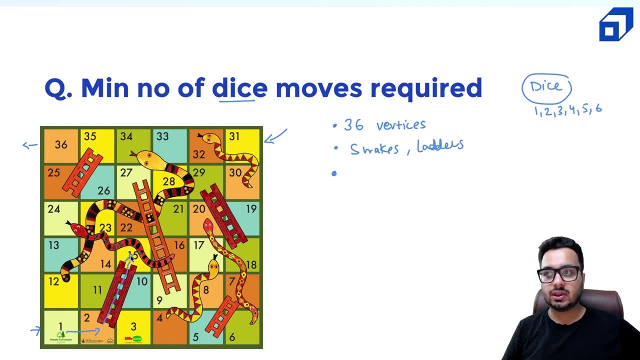 you can reach two, but at two there is a ladder that means you will reach fifteen. so if i talk about this edge- there is an edge from to 15 in this graph- then if at 1, if you throw a dice 2, you can reach 3, there is an edge from 1. 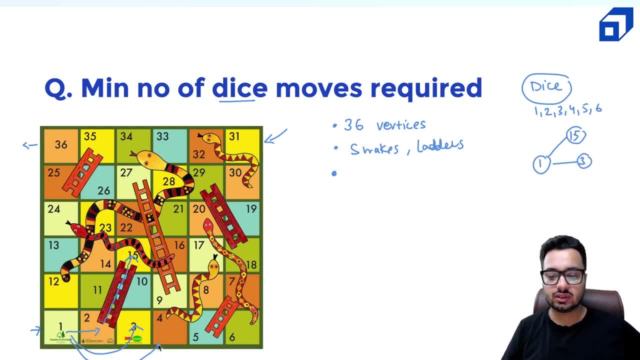 to 3. also, if you throw a 3 on dice, you can reach 4. that means there is a edge to 4 as well, and all of these edges are directed edges. and then, if you throw a 4, you will reach 5, but on 5 there is a. 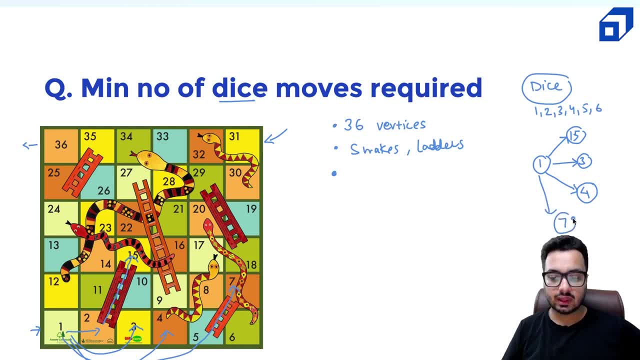 letter. so that means the edge is from 1 to 7. right, and if you throw 5 you can reach 6. that means there is an edge from 1 to 6 also right now. if you throw 6, you can also reach 7. that means it is the. 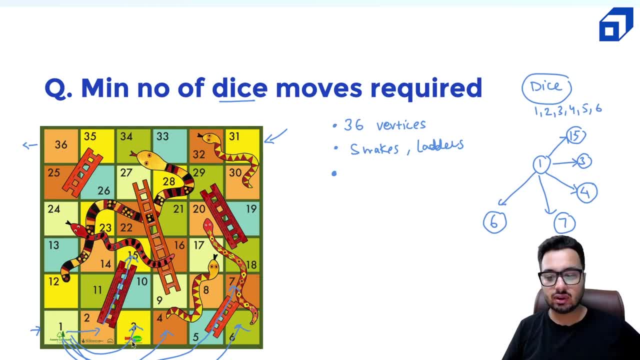 same edge. we will not count that edge again. again starting from 2. so 2, there is a letter, so we do not need to do anything. then you would go at 3. so from 3, again there are edges. so there is an edge from 3 to 4 if, if you see carefully, 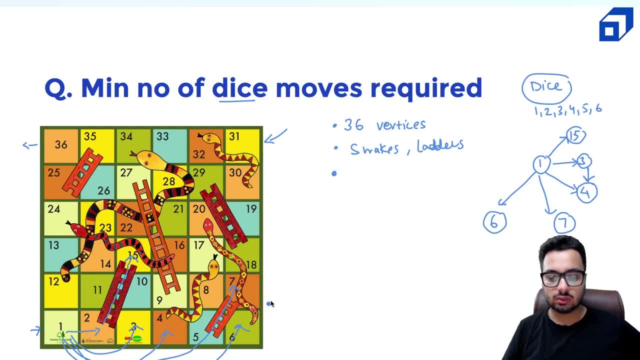 3 you can go to 4, and so on. from 3 you can go to 7. also, from 3 to 7, there is an edge, and so on. that means how many edges i have. so i have approximately 6 edges, starting from each vertex, from approximately 6 edges from each vertex. okay, if the vertex is v. 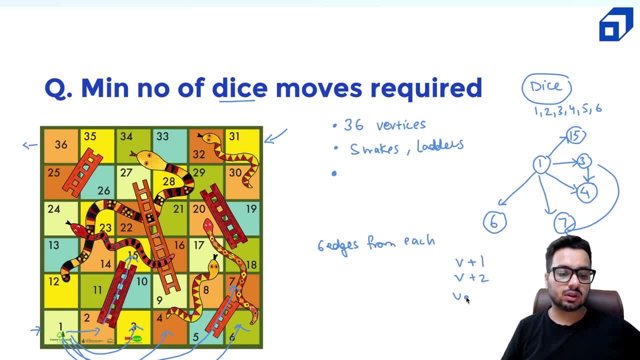 i can go to v plus 1, i can go to v plus 2, i can go to v plus 3, v plus 4, v plus 5. this would have been the case if there was no snake and no letter, but now what is happening is. 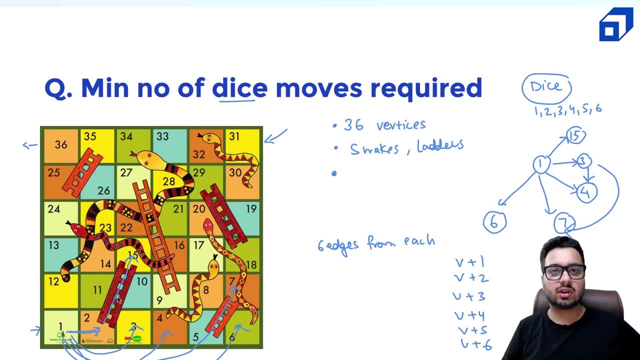 suppose i go to v plus 1 here there is a starting point of the letter. so that means i will reach at some other position. so that means there might be a factor which will add up or which will be subtracted and that vector will come from if there is a letter at that position or if there is a 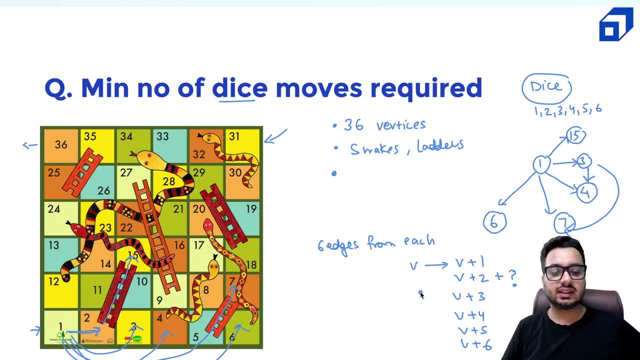 snake at that position. right, that is what i am saying: that it is an example of a directed graph. it is an exam. is it a weighted graph? the answer is no. it is an example of unweighted graph. that means all edges are equal because the cost to 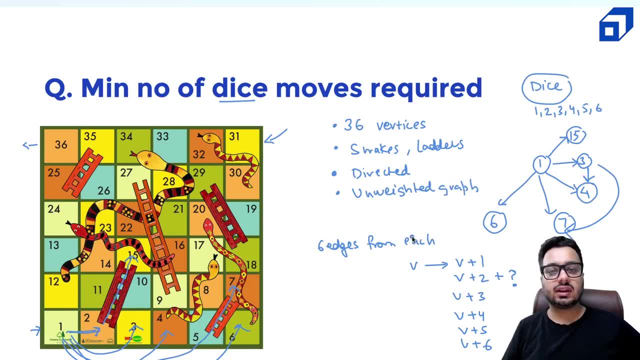 cover in any edge is dice throw. so it does not really depend what number you throw on the die. each move is counted as one throw right. so if you analyze carefully, you will see it. it becomes an example of a directed unweighted graph. and if it is unweighted graph, we can use the bfs shortest. 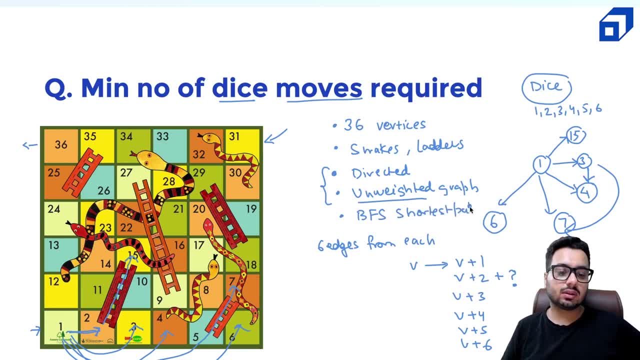 path algorithm to find out how do i reach this node right. so in this case, if i analyze little more carefully, i will see: from 1 i can go to 15, from 15 i can throw 3 and i can reach 18- 18. there is a letter i can. 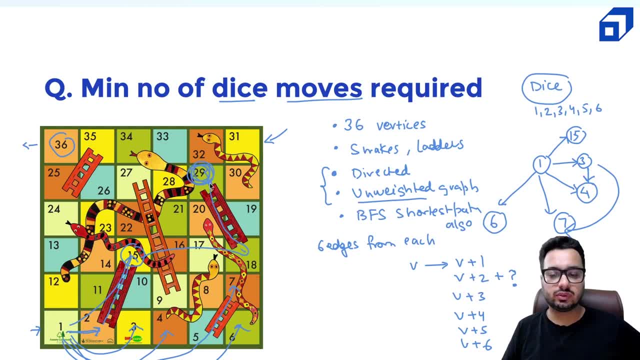 reach 29.. in order to reach 29, i just need two moves. then i can throw one to reach 30 and then i can throw six to reach 36.. so i guess in four moves i can easily finish this game. so i hope the problem statement is clear. now it's your turn to figure out. how do we? 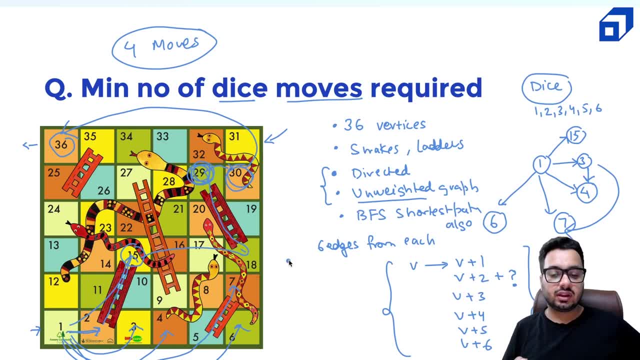 construct such a graph, take input such a graph. so, regarding input, you will be given the number of vertices, the number of snakes, the number of letters, as well as the position of the ladder. for example, 2 to 15, there is a ladder. five to seven, there is a letter right. similarly, 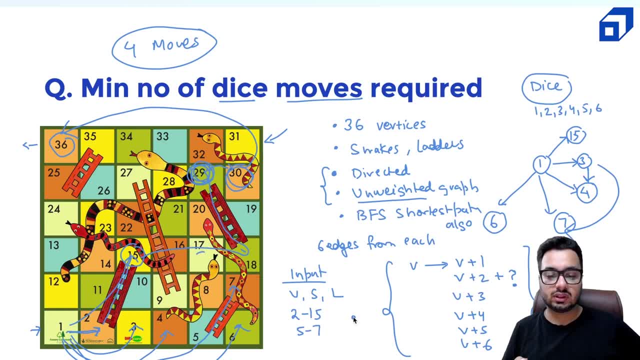 positions of snakes will be given as pairs: 17 to 4. there is a pair, so take a moment to think. how do you input such kind of a graph and how do you make your bfs algorithm run on it? all right, so let us discuss how we are going to build the algorithm. so i have 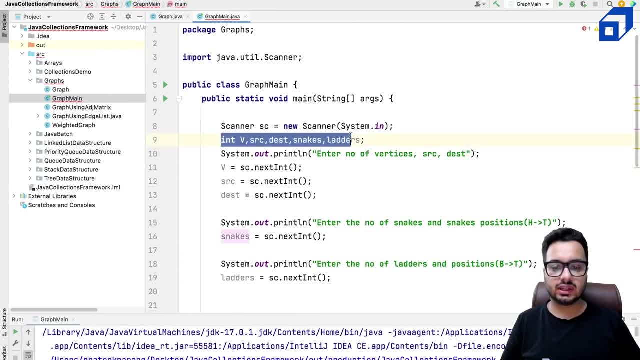 written some boilerplate code. it's not the complete code, so i'm going to read some. some inputs. i'm going to ask: enter the number of vertices, source and the destination. so i'm going to read these three things. after that i will create a graph, since i know the number of vertices right. 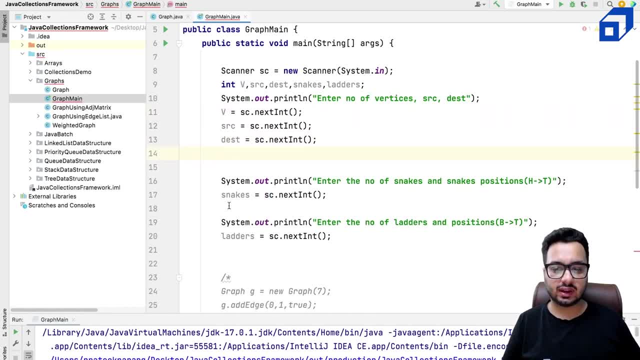 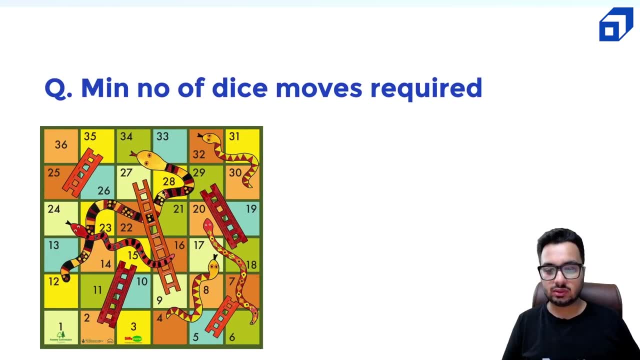 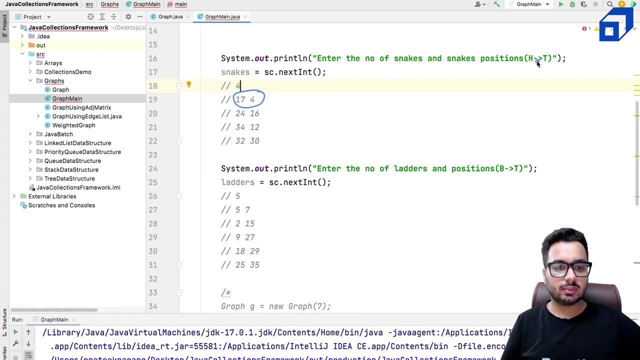 i can create a graph object or i can do it later on as well. that's fine, and i'm going to read the number of snakes and their positions. so in our scenario we have one, two, three and four snakes. number of snakes in my case are four and these are the positions of the snakes: 17 to 4. so i'm 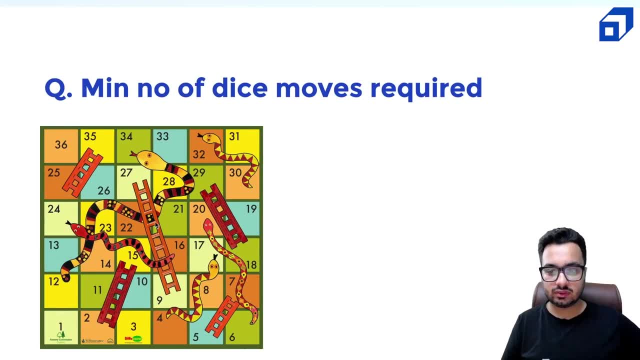 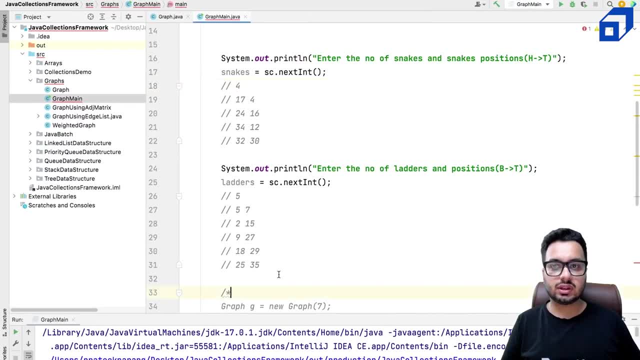 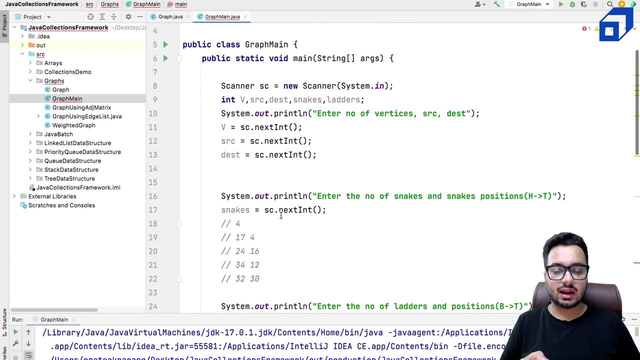 there is a letter. so 5 to 7, there is a letter. so 5 to 7, there is a letter. the question is: how do we like handle this data? what should i do with this data? first of all, i need to read this and i need 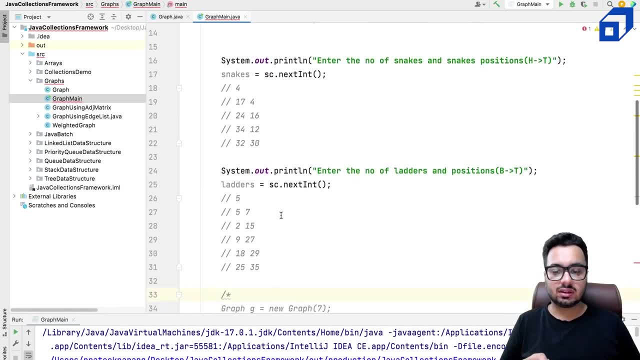 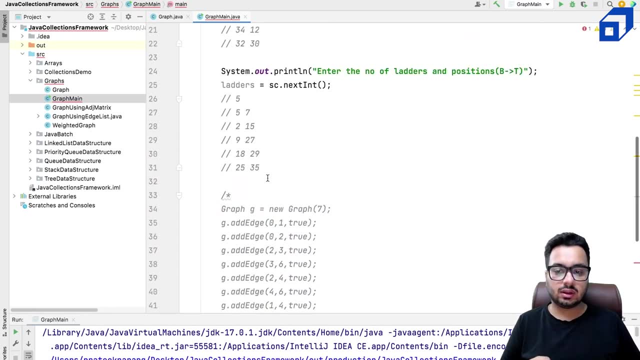 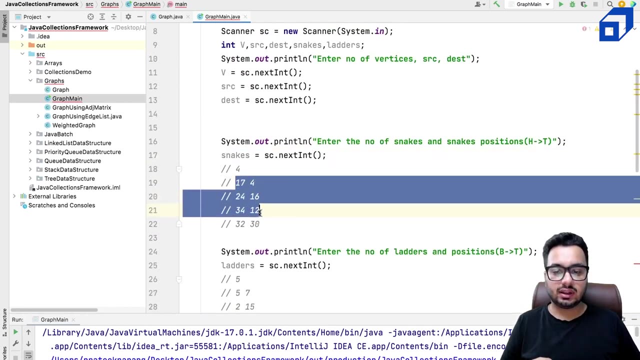 to make sure that this data is used in my construction of the graph. earlier we were creating a hard-coded graph, so we'll not do that thing here, right? so we'll, uh, create our own graph. the first thing is here: i'm just reading the number of snakes. i'm not reading what snakes i 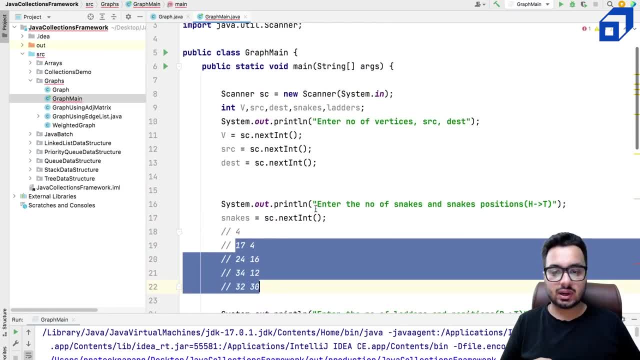 have. so i'm just reading the number of snakes. i'm not reading what snakes i have, so i'm just reading the number of snakes i have. so i'm just reading the number of snakes i have. so i need to implement logic for that. need to implement logic for that as well. right, this part, i'm going to do it right now. so let's. 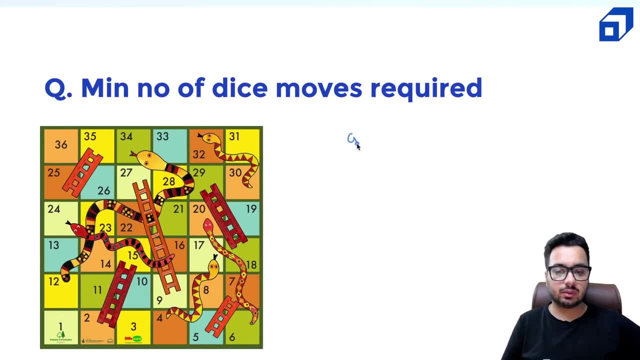 try to understand how we will actually create a graph. so we'll create a graph, object d, and we will, of course, we'll try to add edges to it. add edge now in edge. you need to know that, from where the edge starts and where the edge ends, right and it is a directed edge, so it's not a. 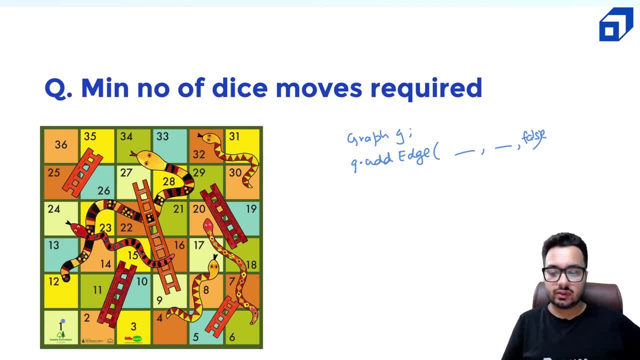 undirected graph. so i will set this third parameter as false. now, if i talk about vertex one- so i told you, from one i can go to, let's say, vertex i- i can go to i plus one, i can go to i plus two, i plus three, i plus four, i plus five, i plus six and plus something right- this value could be. 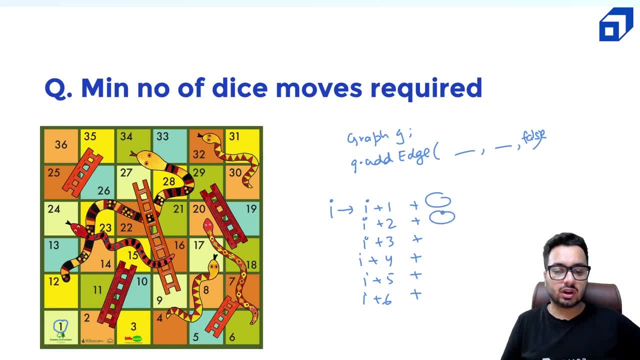 zero. this value could be positive value, this could be negative value. what is this something going to be? it will depend upon whether there is a snake or a letter starting from that position, for example, i plus one, so at two i have a letter which gives me, which actually takes me to the next position, so i 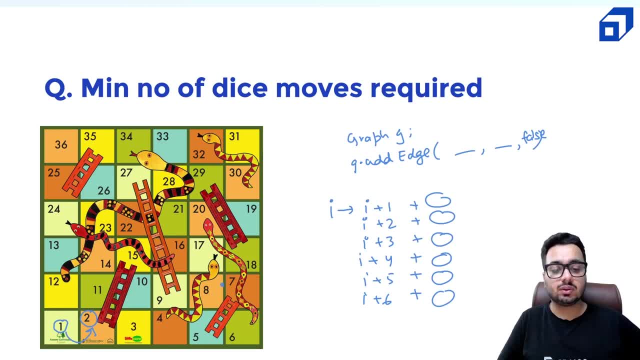 have a letter which takes me to 15, right, which i, which is actually taking me to 15. that means i'm getting a jump of 13, right? so, for example, if i is one, i take a move of one, i reach two and two. there is a letter which is giving me a jump of 15 minus two, right? so basically, there is a letter, so the 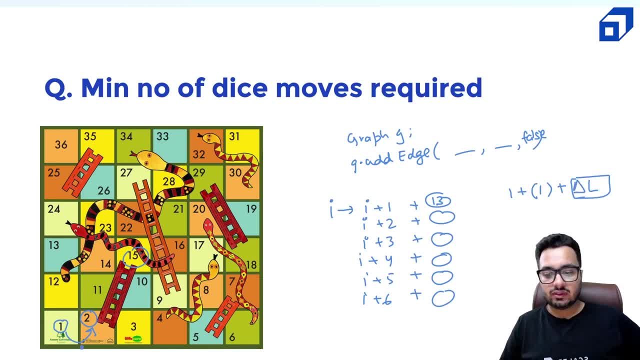 delta that is given by the letter right. so if i go to, let's say, uh, i, i plus three, so there is no degree of delta in here. so i go to, i plus four, i reach five. at five, i actually reach seven. so this delta is two. how do i compute this delta, this delta? i have to compute and store it in a array. 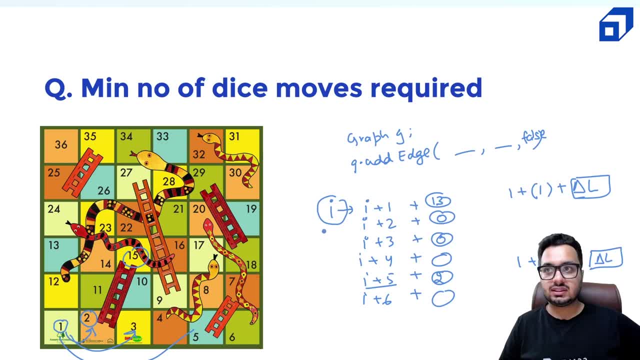 i have to compute and store it in an array, so that means in an edge. this becomes a starting point and this becomes the ending point of the edge. so this delta is very easy to compute. for example, you are given there, there is a letter from 2 to 15.. you can easily say, okay, i'm going to store it in some. 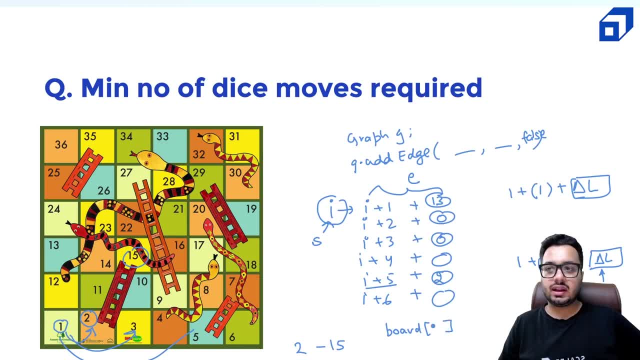 create a board array. right, so it's. it's a 1d array of 36 positions and in each position i'm going to store a delta. if someone says, okay, there is a letter from 2 to 15, that means at the second position in this array, i can store 15 minus 2, that is, 13.. at the second index in this array, i can. 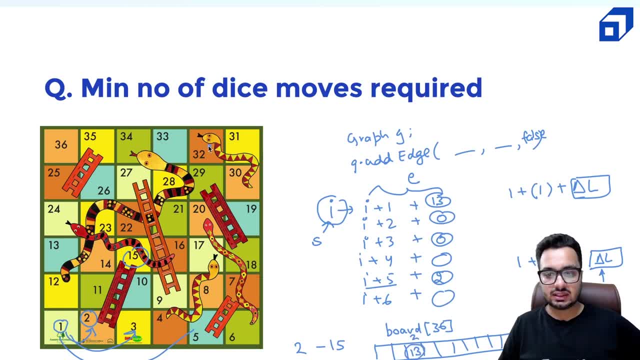 store 13.. so if there is a snake at, let's say, 32, which takes me at 30. let us assume this index is 32.. so at 32 i get a delta of minus 2.. so if i reach 32, effectively i reach 30 to 32 minus 2.. 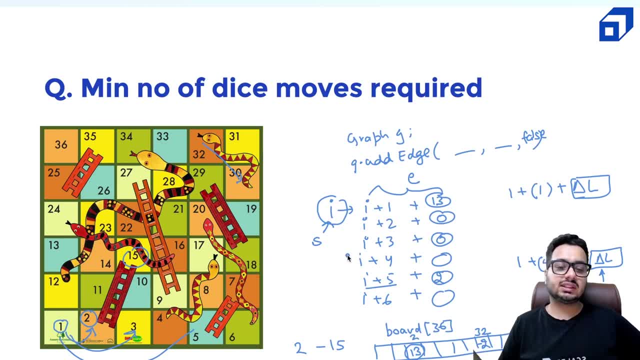 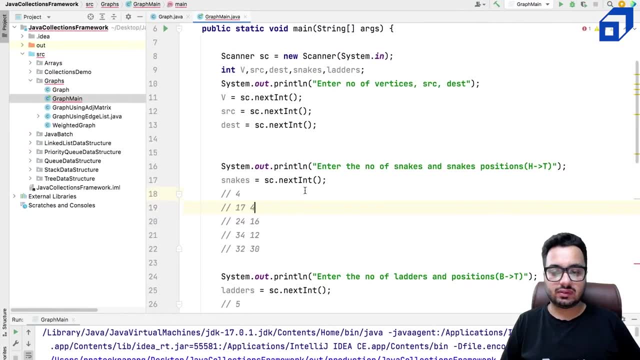 this is how i am going to do it. once all the edges have been inserted into the graph, i can easily run bfs on it. so let us try to insert all these edges into our graph. what i'm going to do? i'm going to run a loop. let's say for i equal to 0, i less than snakes, i plus plus. 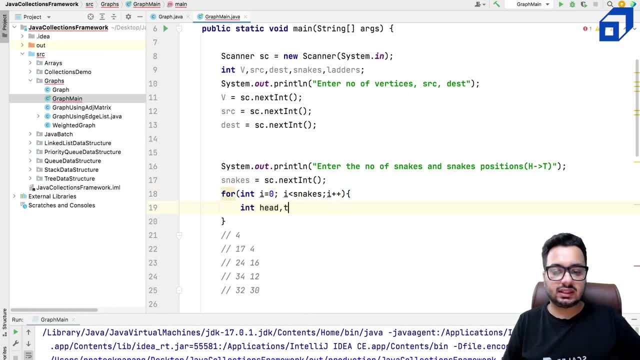 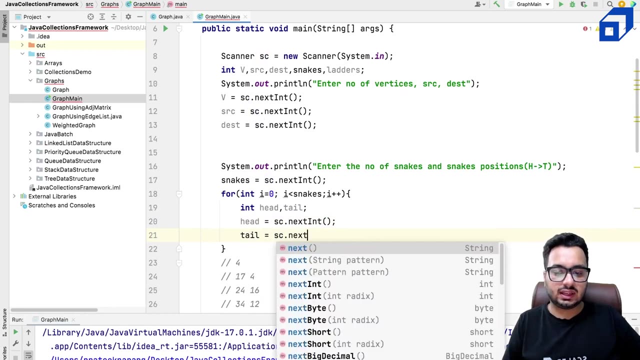 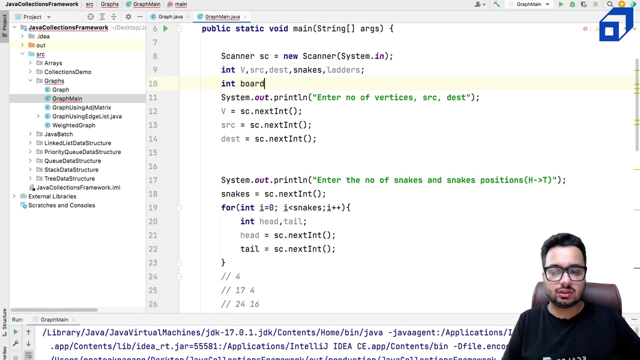 i can show: snake has a head and snake has a tail. i'm going to read these values so i can say: head equal to scanner dot extent. tail equal to scanner dot. next int. and i'm also going to create a board array so the board array can be created here. so int, board and this is equal to new, and how many. 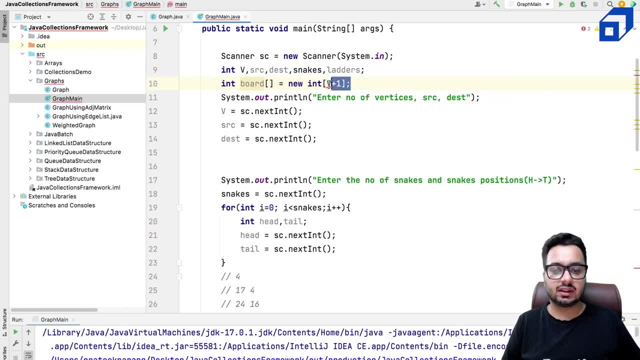 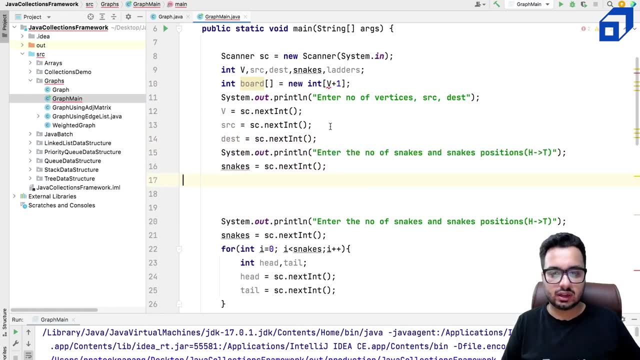 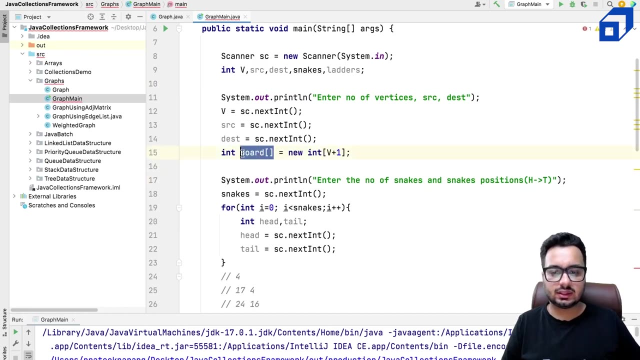 i'm going to do v plus one, because it is a one base indexing here. so i've created a board array. oh, i have to move this code here because v is not input yet, so this board array will come here, or you can do it like this: that's fine. that's fine, board array is now created. so now, when, when i'm 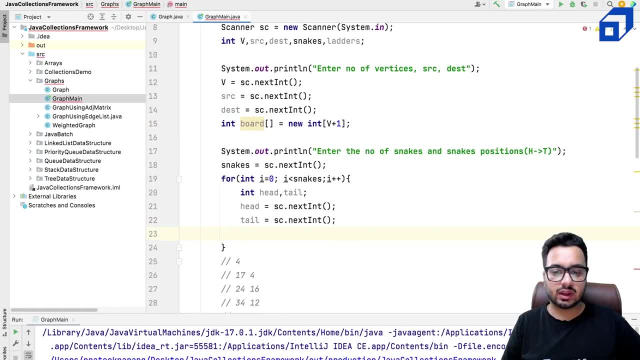 reading the snakes right. so i have to update the board array so i can say, okay, board off, head in to buy it from the head. right, the board of head will store a value that is equal to, because now it is giving you a decrement. so from 17 you are going going at 4, right, let's look, look once again. 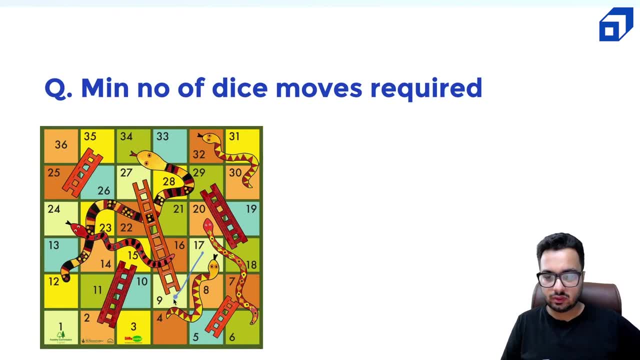 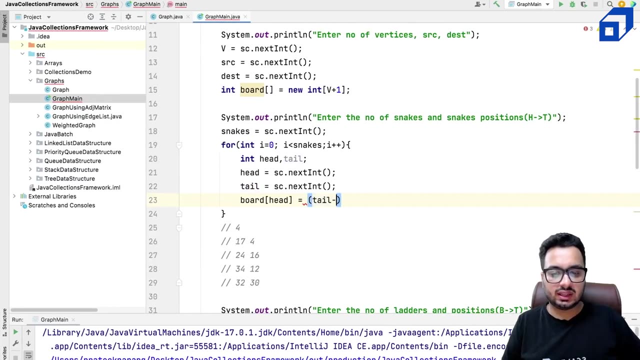 from 17, you are going at 4.. the board of 17 should say that my value is nothing but 4 minus 17, so this value should be minus 30.. this is how it should be, so it should be equal to tail minus head. so tail is a small value, head is a large value, so this value needs to be. 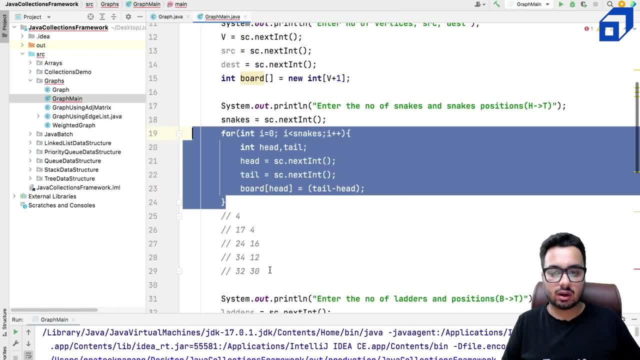 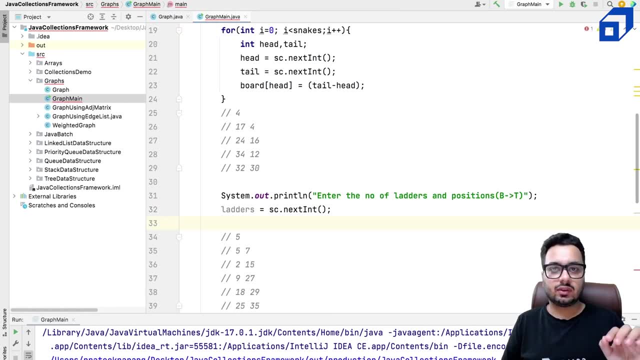 negative. this will update the board array for snakes. similarly, we need to update the board array for letters and we will utilize this array while constructing the graph. i will show you how make a similar loop. i have the letters instead of snakes here. i will have letters. now the letters. 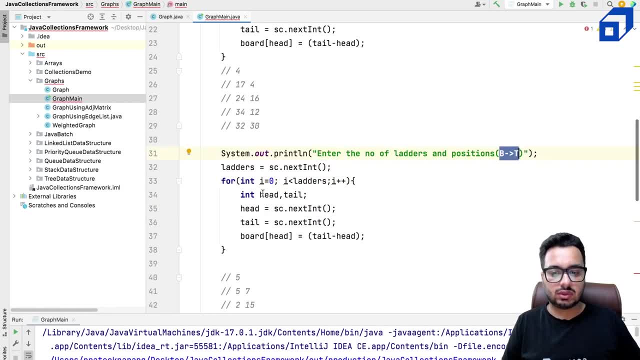 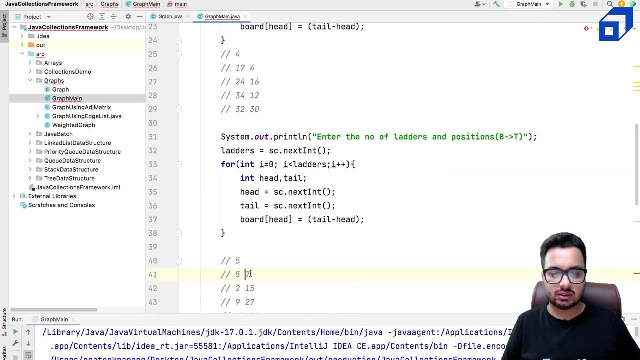 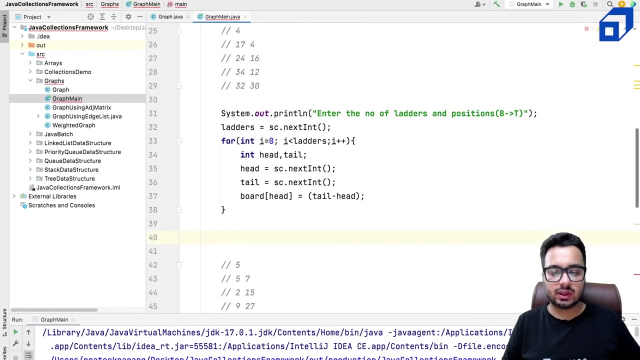 are given in this fashion: bottom to top. so letter also has a head and it also has a tail. so tail is this number is smaller. this number is bigger. tail minus head would be a positive number here. that is fine. i think board array looks fine so i can just display you the board array as well. i can say s out, it is dot. 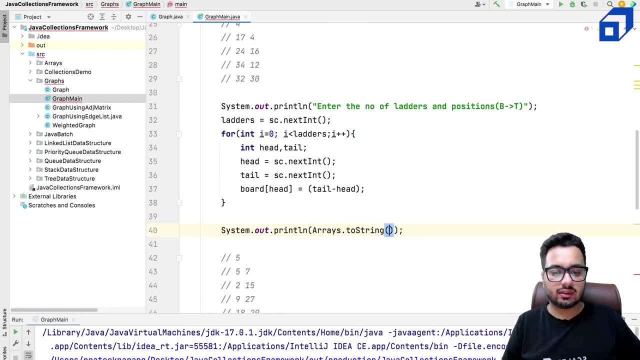 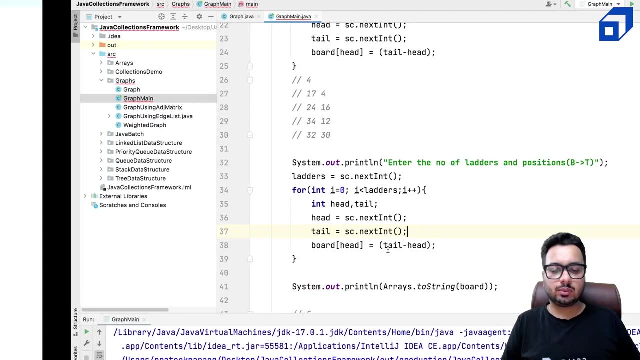 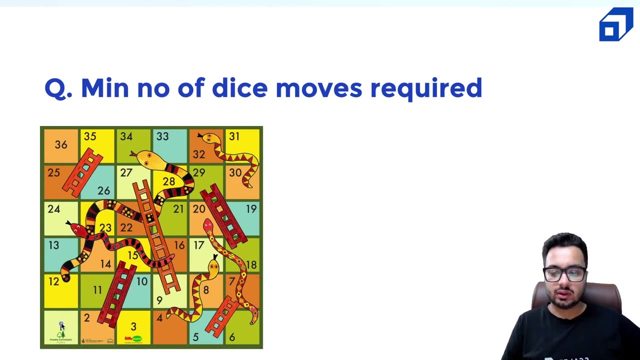 two string and i can give the board array. now i have this board array, i have these delta increments. again, i need to figure out how do i insert all the edges. now that thing is fairly simple. you need to go to every vertex and create the next six edges that will start from that vertex. for example, if i start from five, or if i 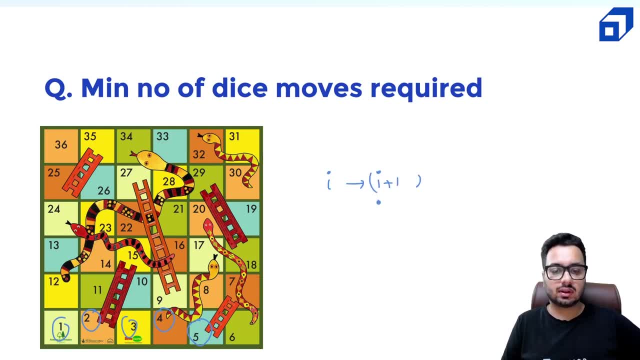 start from i, i can go to i plus one plus board of this position that you have reached. if you do five plus- let's say some number, five or five plus four, you reach nine. but nine is not the end position. you actually reach 27, right, i plus two plus board of this position. i plus three, up to up to i plus six, basically. 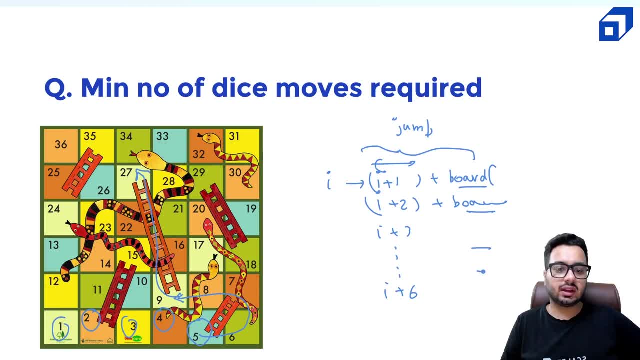 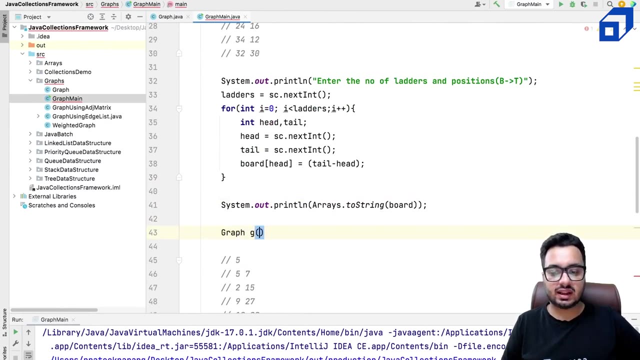 from ith node where i can go. so here i'm going to use the board array to decide where i can actually go. so this will be board of i plus one, board of i plus two, and so on. so let's see here as well. let's create the graph now. so i have graph g, how many vertices i have. i have v vertices, so i'll 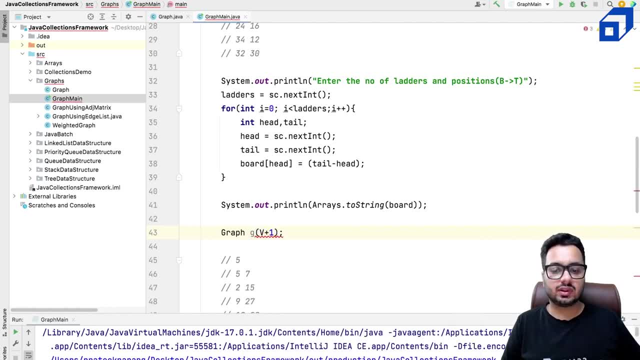 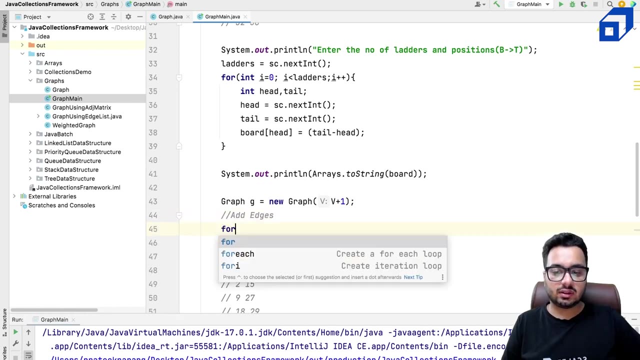 just keep v plus one because it is one based. so we we are also adding zero here. this is equal to new graph, new graph of v plus one vertices. all right, i have to add edges, right, so i can do okay for int. let's say: source which starts from. or let's say: 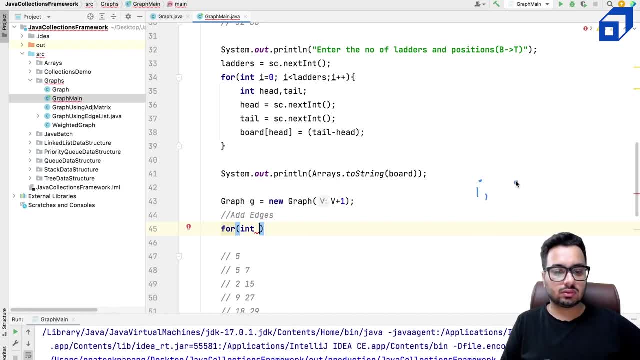 i'm going to add edge from i to something, so i do some j. okay, so if i goes from, i can start from source, which is one, the smallest node i can go till less than destination. that is my last node. i plus, plus, so i'm going at every node. then i can throw a dice at every node. i can throw one, two. 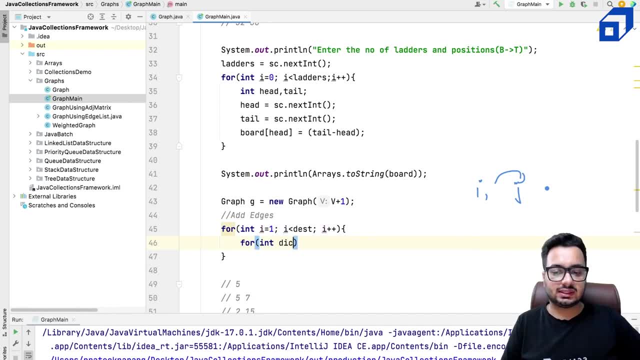 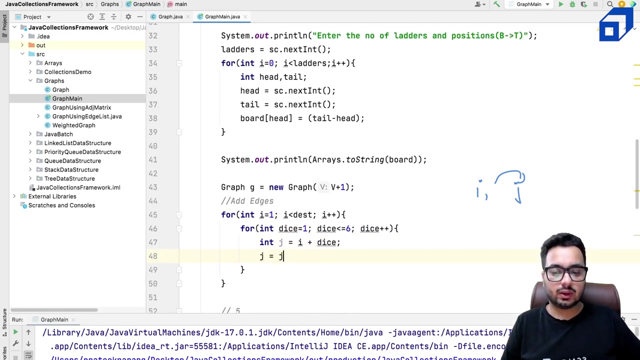 three, four, five, six. so i can throw a dice, dice can take a value, one. the maximum value dice can take is six and i can say dice plus, plus. so what is the node? that where i'm reaching the jth node is, uh, i plus dice. right, but this is not final. i also have to add delta so i can, okay, j equal to j plus. 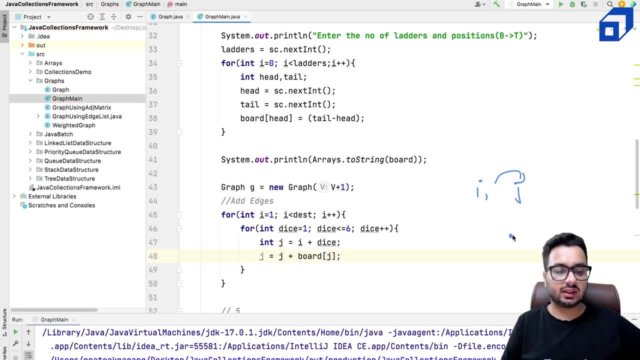 board of j in this value. what i'm saying is: from i you throw a die, you reach i plus dice. now, at this position, it is possible that there is a ladder. the ladder gives you a jump of 13. so you have to add this vector also. that is stored in board of j. but if there is a snake that takes you down, so you 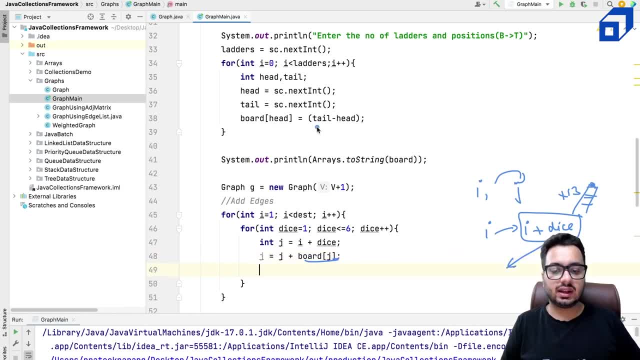 have to decrement this value. also that addition subtraction is already handled in the board array. if j is less than equal to destination, that means i do not want to add any edge. that goes out of the board. so i can say g dot add edge. so u is in my i. 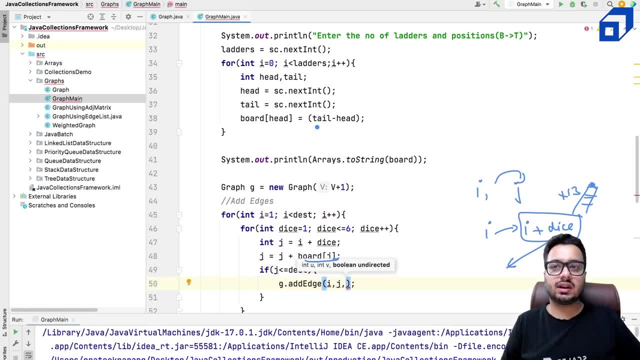 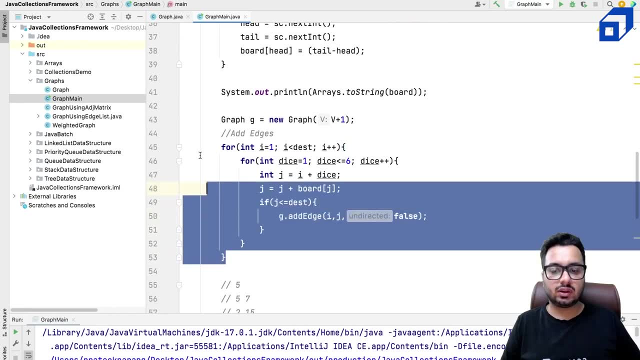 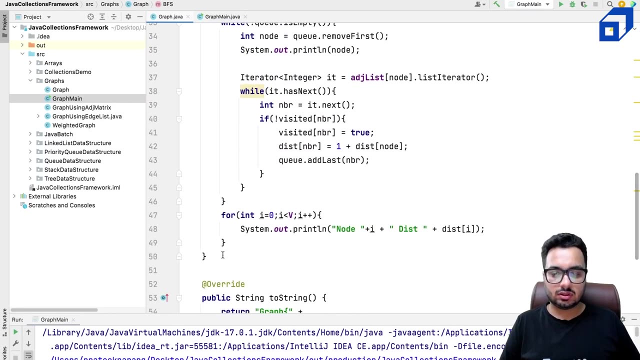 j and it is a. it is not undirected graph, so this value is going to be said to be. this completes the graph creation process. now what we need to do? we need to run bfs algorithm on it. so, as you know, we have already implemented the bfs algorithm. i'll just copy this code and tweak it a little bit so that we can do. 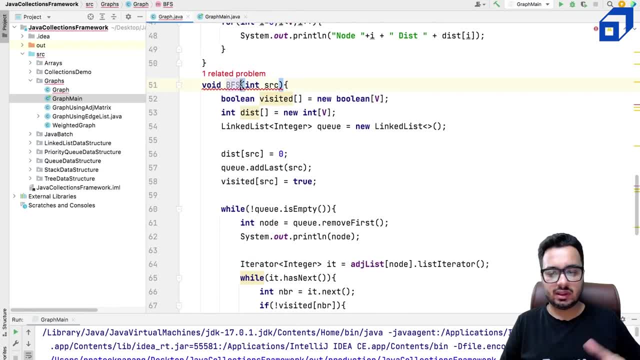 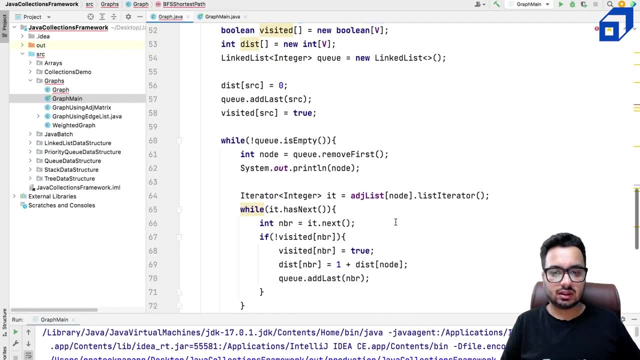 it. for this particular problem i can say bfs, dot, testpath, so in this case i am getting sourced, i'm also getting thisお願いします. i could change the algorithm along with the a uh without training of also getting the destination. so if the user is interested in finding out, uh. minimum number of. 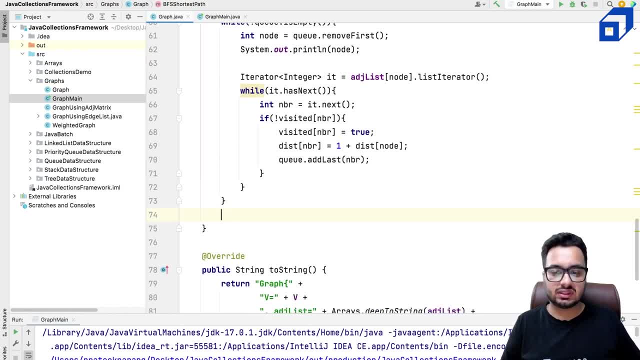 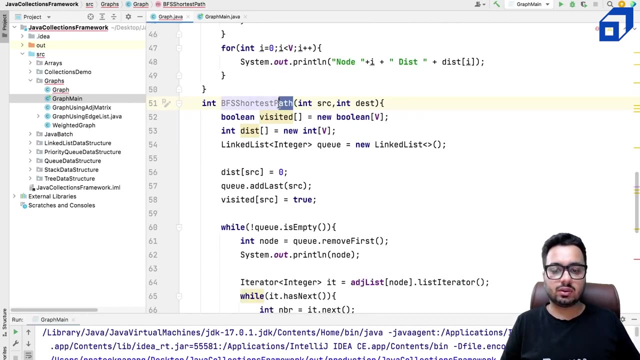 moves. so you do not need to print distance every node. you can simply return the distance of destination and you can change the return type to integer. this can be done. now one thing might ask is: user might ask you to give the path. also, as i discussed with you, along with the 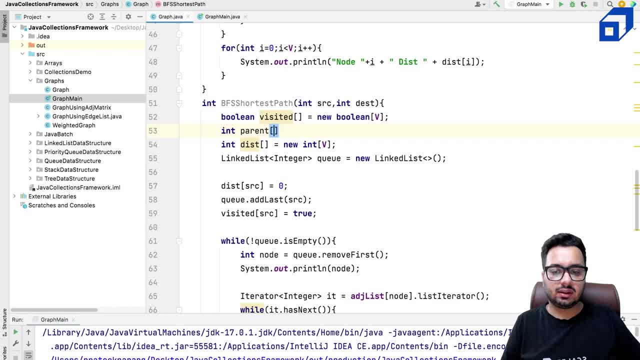 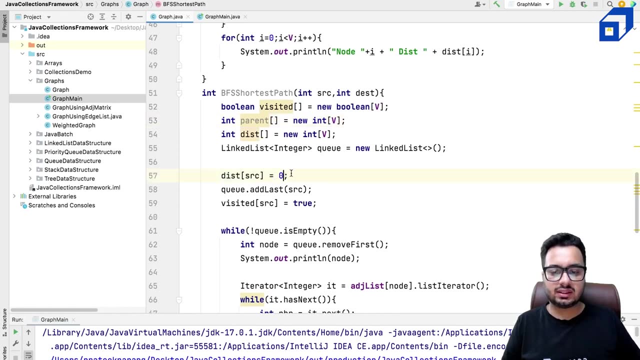 visited array. you can create a parent array as well and you can say: okay, this is equal to new, new integer of v. and here you can say: okay, for first node, that is my source node, the parent is, let's say, minus one. so parent of source, this is minus one, or you can set this is: 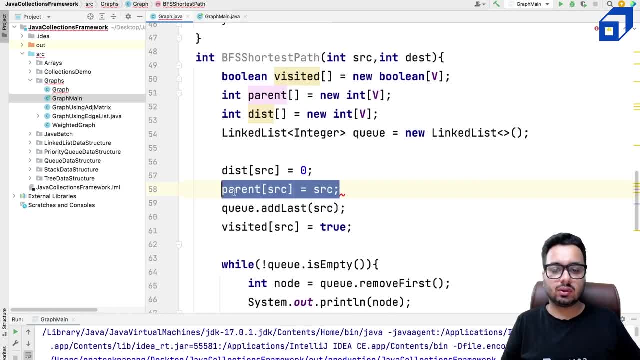 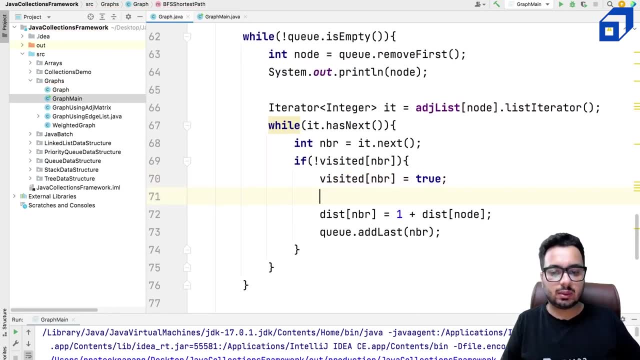 the source itself, something like this, so that you can know, right right now i can. i'm just saying this is going to be a parent of source, so i'm going to say parent of source, so i'm going to be minus 1 and whenever you visit a node, you can set the parent. parent of neighbor is going to be. 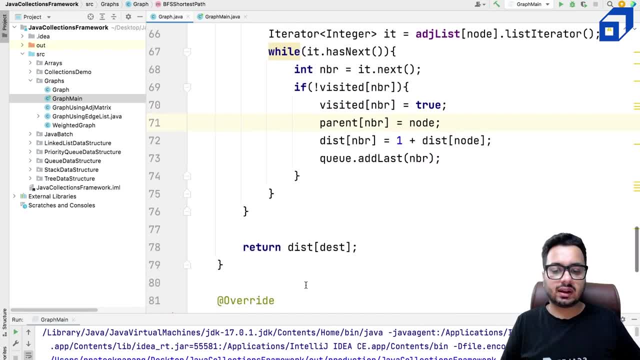 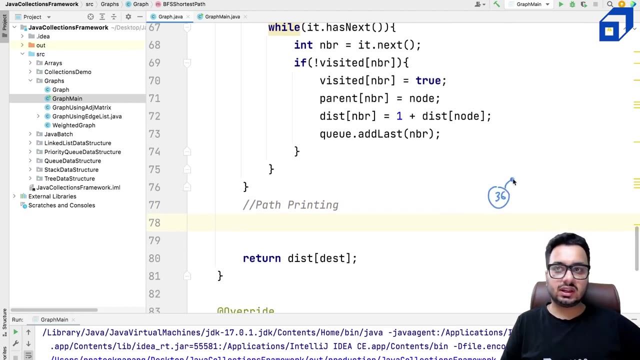 the node. now, as i told you, you can backtrack and you can find out the complete path as well. let us discuss that thing as well. if you want to do the path printing, that is fairly simple. you can start from the destination node. let's say 36- now 36 nodes from where i was visited, so maybe the parent 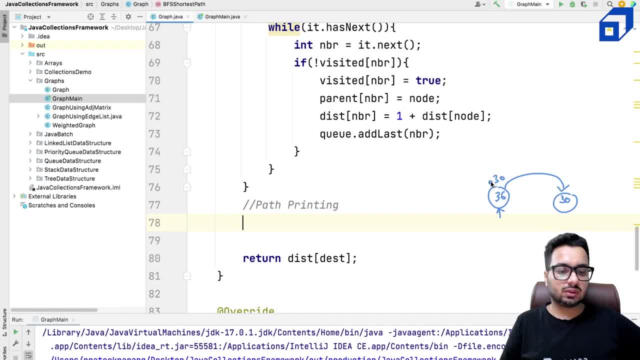 of 36 is 36, so now i can find the complete path and i can also set the parent of the destination node Right, So I can start from this node, reach this node again, ask the parent: go back, go back. 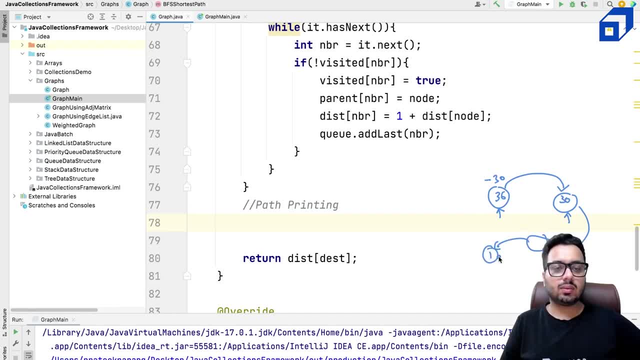 And so on. I can trace the path until I hit one or minus one, something like that. So I can define. I take a temporary value which is destination, And I can say while parent of destination or while parent of temp is not equal to minus. 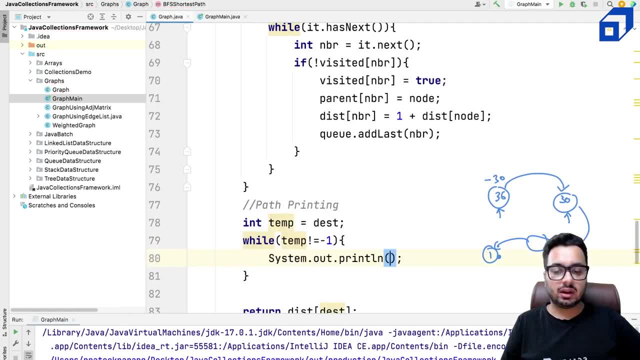 one. what do I do is okay, fine, I will print out the destination. I will print out the temporary node. So basically, what I'm saying is: the temporary node is this. temporary node is 36.. I will print it out and I will go here. this will become the new temporary node. 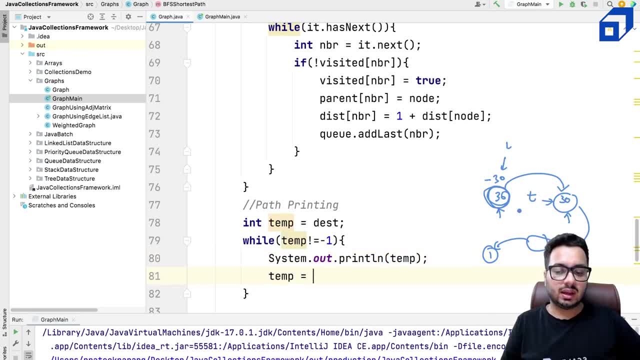 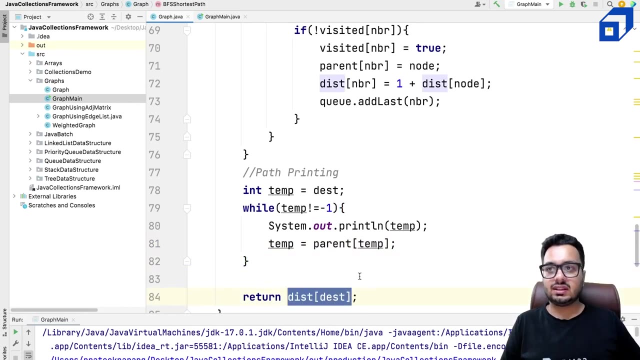 But how do I update this temporary node? fairly simple: temp equal to parent of temp. at every node I take it back to the parent. So this is basically going back to the previous node in the path, how it was discovered. then I'm saying return the distance of the destination. 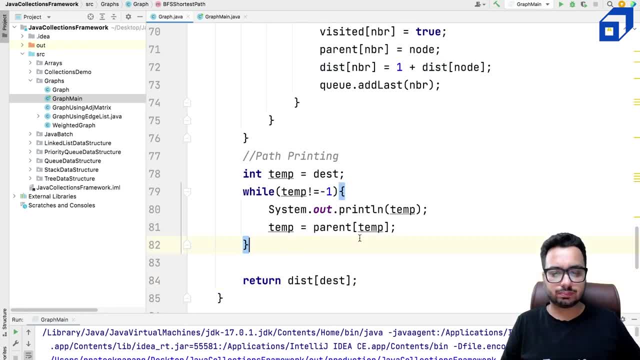 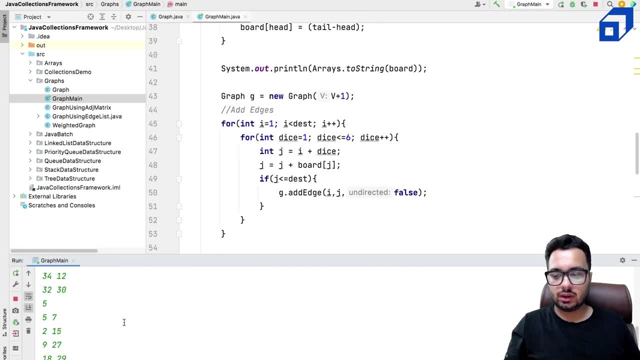 Now let us go and run this code. I think it should be fine. Yeah, it seems fine. Let us try to execute the code. So I've given the input, I've just combined the input and I'm giving it, but now I'm getting. 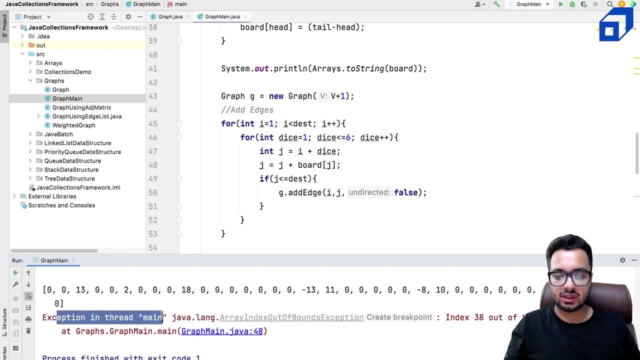 an error. actually, I'll tell you what. what is there? So it is saying exception in thread main index, that it out of bounds. So in main, this is the array, So this is going out of bounds. Why this is happening? Because if you add something to, let's say, node, 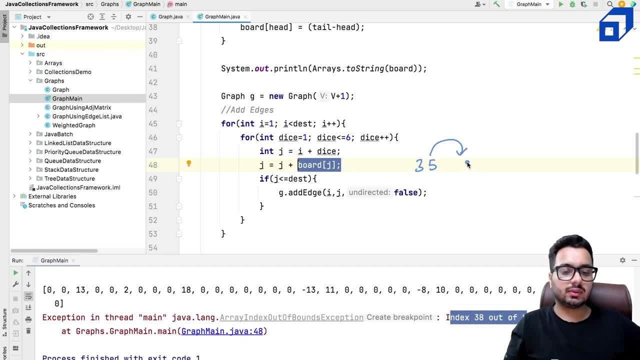 Okay, 35 years. okay, I will take a jump off three, you will actually reach 38. actually, I'm checking it here. So instead, this check should be done here, right? So when I'm doing this value, when I'm computing this j, so I should do this thing here. 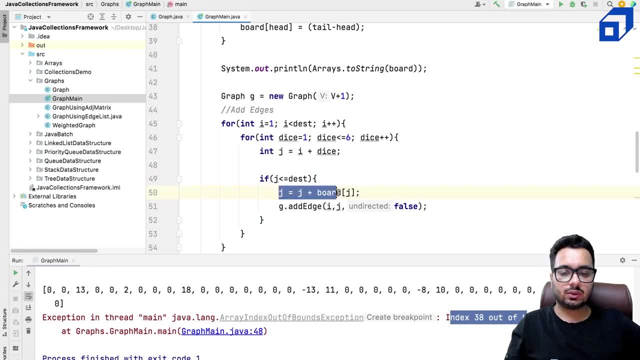 If j is less than equal to destination, then I should do j equal to board of j And again I should check if j is. you can do it here, That is fine. So if j is now less than equal to destination, Then you can actually add that edge. I think this would be okay. 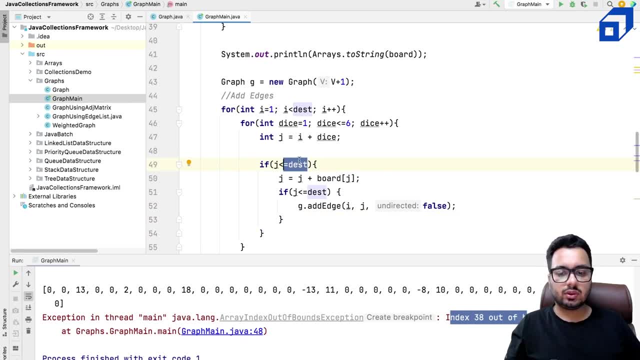 Or you can do two conditions here, right? You need to check that, see what is happening. is I added something here? I said, okay, 35 plus two or 35, let's say 33 plus two. okay, And suppose there was a letter here, right? 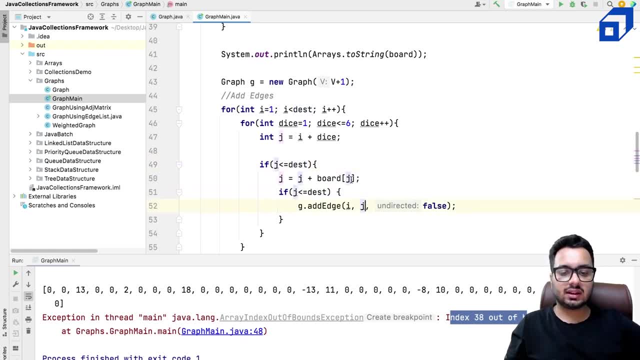 It might. it's not going to take you out. But what I'm checking is that when I'm adding this value board of j, a must be less than destination, And when I'm adding the edge, that edge must be less than destination.